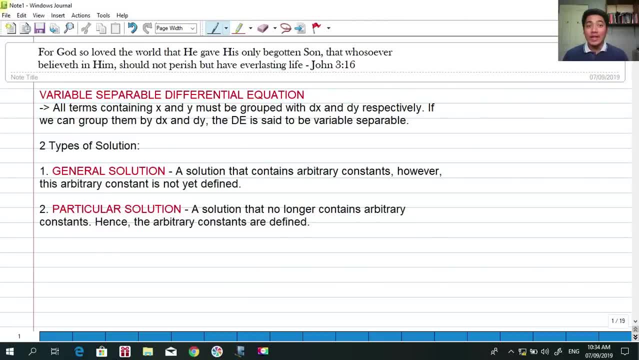 Hi, so for today, we're going to talk about variable separable DE. Okay, so this is a next topic, when you are already done with families of curves, and we're going to solve some problems involving variable separable DE. I have here about eight examples so that we could at least 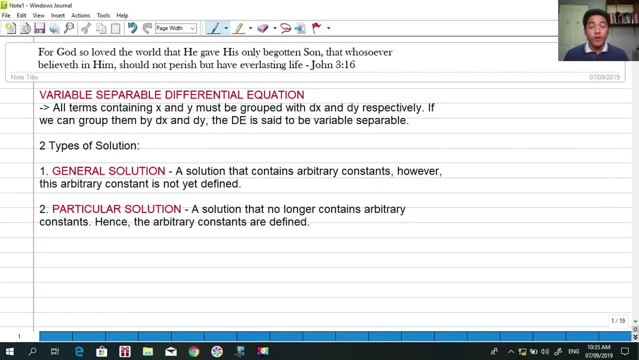 master the solution of a variable separable DE. Now, what is a variable separable differential equation? So we can say that a DE is a variable separable if all terms containing x can be grouped with dx and y can be grouped with the dy. So all terms containing x and y must be grouped with dx. 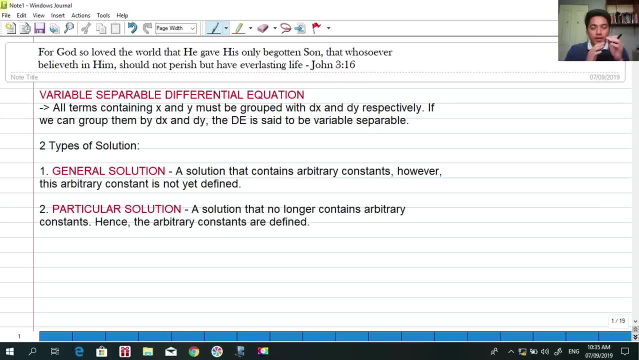 and dy respectively. So if we can group the functions of x with dx and the functions of y with dy, then the DE is said to be variable separable. So now we have two types of solutions. Okay, so number one: 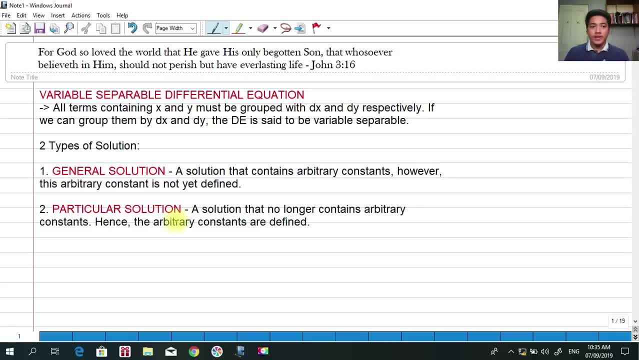 we have the general solution and a particular solution in DE. So a general solution, a solution that contains arbitrary constants. However, those arbitrary constants, or this arbitrary constants, is not yet defined. In our previous discussion of differential equations, our main goal in the families of curves and in the 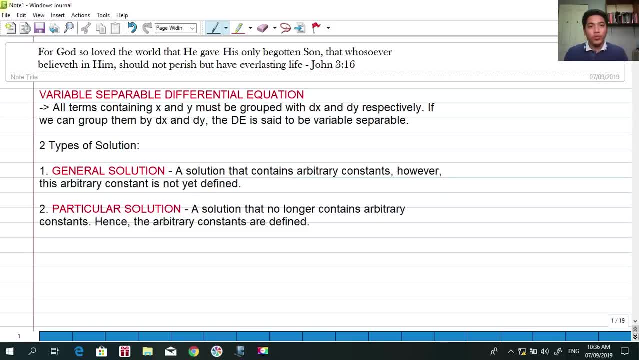 elimination of arbitrary constants we need to eliminate. we need to come up with a differential equation that does not longer contain an arbitrary constant. Here, in the solutions of differential equations, such as variable, separable differential equations, we're going to come up with a constant. 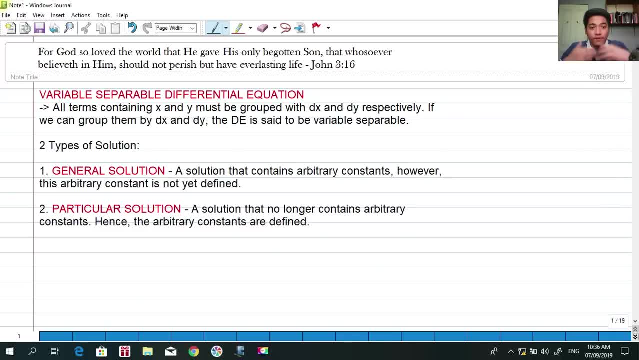 And that constant is actually can be defined and not yet defined. So if the constant is not yet defined or its value is unknown, that is what we call the general solution. Okay, we have here the particular solution. So, particular solution, a solution that no longer contains arbitrary constant. 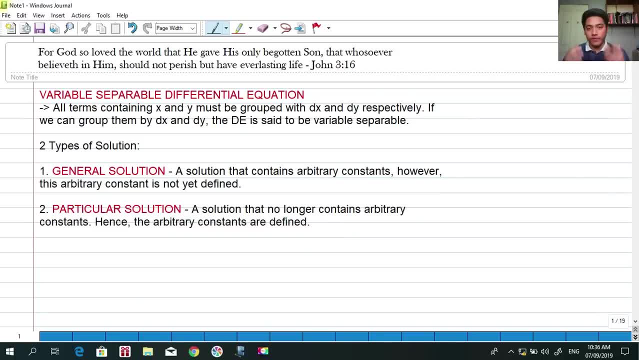 meaning the arbitrary constant now here are defined, It means that it has already a value. You have already computed for the value given a certain condition in the differential equation, Okay. so again, if we are solving differential equation, our goal here, okay, is to eliminate the DX and DY, So in our families of curves, 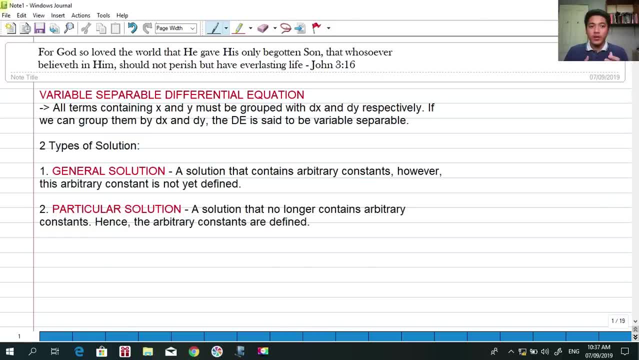 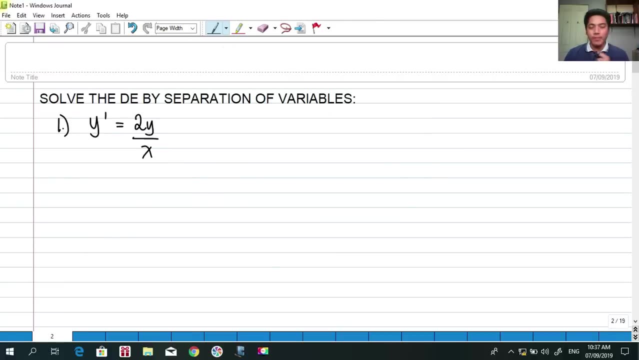 and arbitrary constants. again, we need to eliminate the constant Here. our answer should have constants and we have to eliminate the DX and DY, or actually the derivatives. Okay, so let's get started. So for number one, solve the DE by separation of 2x and 2y. 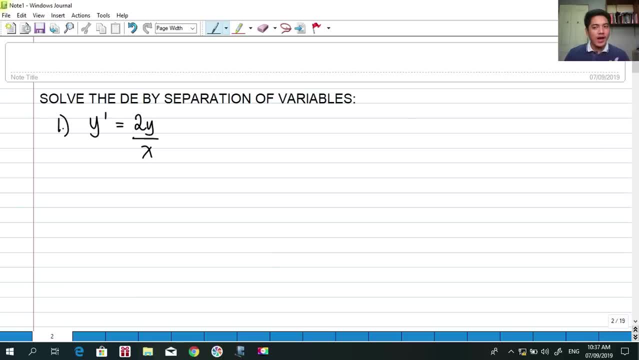 variables. okay, so this is a very easy example. okay, we know that class that we have dy over dx, y prime is equal to dy over dx and that is equivalent to 2y over x. okay, separation of variables. separable: de says that if we can group all the d? y's into the y and all the dx into the, 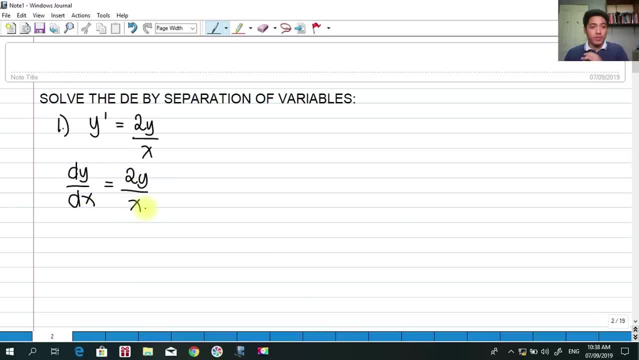 x. okay, that is said to be a variable, separable de. so if i'm going to cross, multiply these two, so what will happen? i will have dy over 2y is equals to now dx over x, as you can see now here on the left side of our equation, dy of our function of y. okay, all terms of y is grouped. 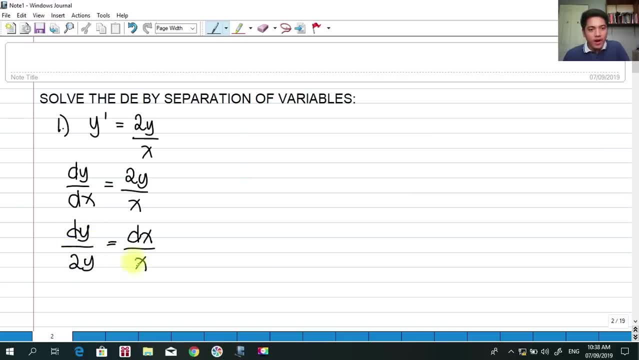 into dy. okay, and all functions of x are now grouped into dx in this example. so what are we going to do here is, in order for us to get the solution upon uh, grouping these variables into its certain or into his uh respective y, dy's and dx. what are we going to do? 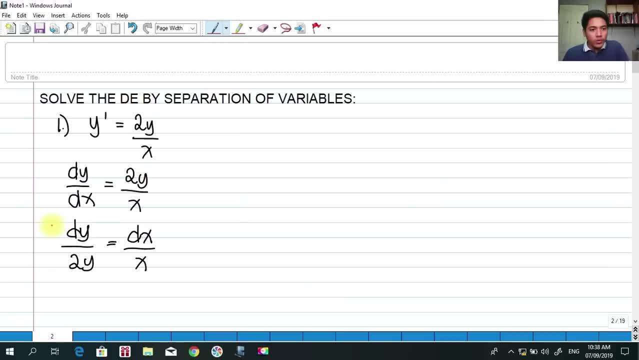 next is: actually, we're going to integrate both sides of the equation. okay, that's right. so, upon integration, we all know that whenever- okay, whenever- we perform integration, integrals, there is always a plus constant. so that is what we are trying to do here. okay, so we know that if we integrate this, we can factor out one half, because that is a constant outside. 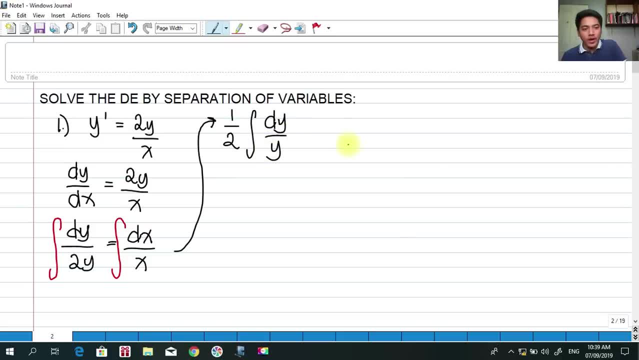 of the integral sign. we have dy over y and we have the integral of dx over x, okay. so if we integrate dy over y, that is simply ln of y, okay, and the integral of dx over x is simply what ln of x plus the integration constant c. so in our study of variables parable, we can choose. 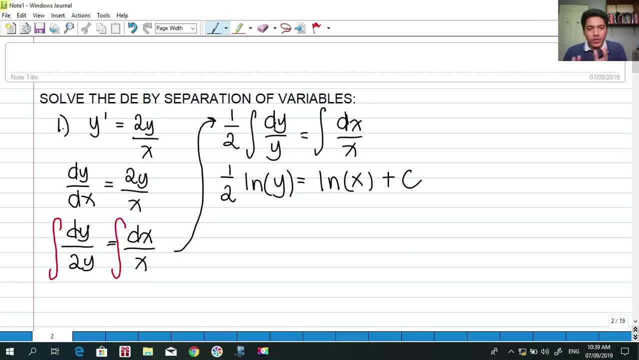 where we are going to write c, but actually we can always attach this into one of those integrals plus c. okay, so how do we do this? how do we do this? so, actually, continuing this by properties of logarithm, we can multiply. okay, we can multiply. 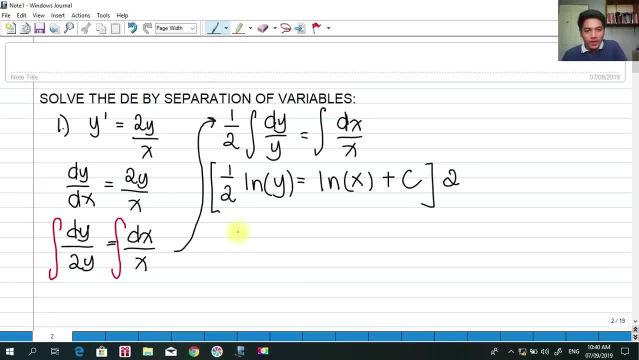 both sides by 2 to cancel the one half. so we have: ln of y is equals to 2 ln of x plus twice the c by 2 times c. remember here in in de the constant, twice a constant, still we can label it as still the c, because twice the constant is still the constant. okay so, and we know class. 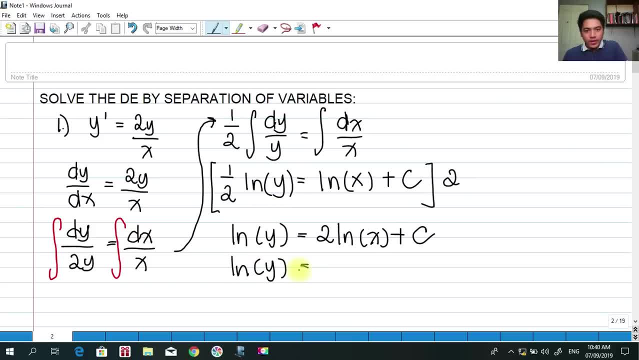 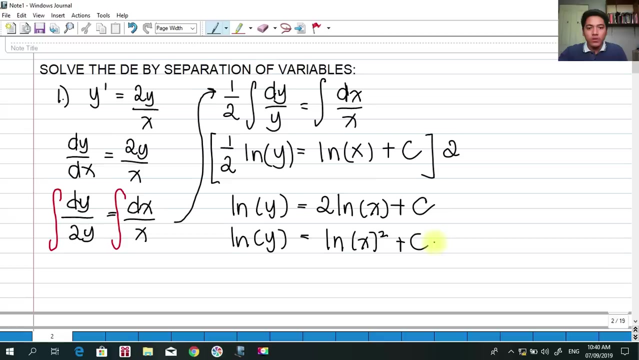 that by the properties of logarithm these two ln. x can be written as ln. okay, oops, ln, ln of x squared. so whatever the coefficient here, you can always rewrite it as the exponent inside the logarithmic sign. so we have plus c. now our main goal, since both the y and both the x are. 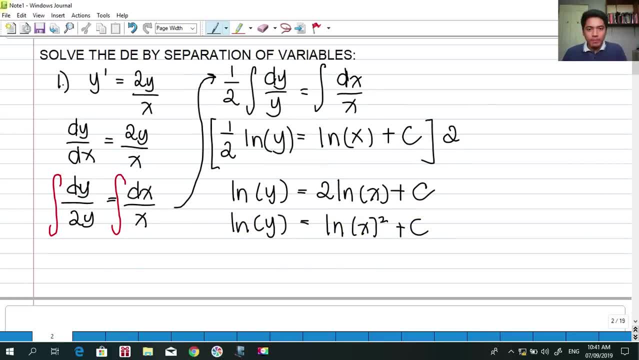 in terms of ln. i could simplify them by: i could eliminate the ln sign, the natural logarithm sign, by actually what? raising them both into? e okay, both sides of the equation. so whatever you do on the left side of the equation, definitely you're going to do on the right side of the equation. 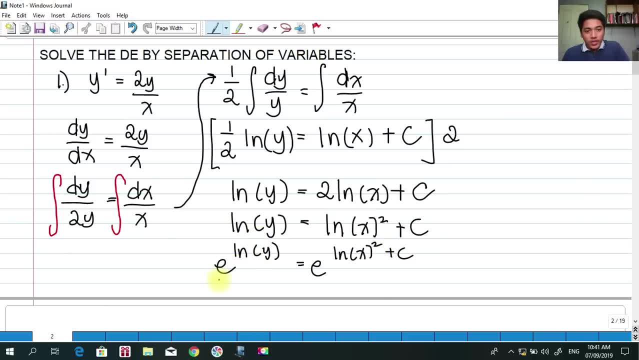 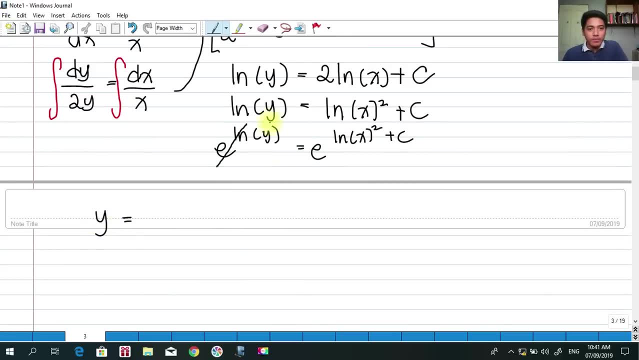 so that e raised to ln, this would be cancelled and the left side of our equation will simply be y. okay, will simply be y. that's a proper e when we raise ln to e. so whatever it is inside the ln, that would be the the result. okay, and here, by properties of exponent, we have eln x squared. 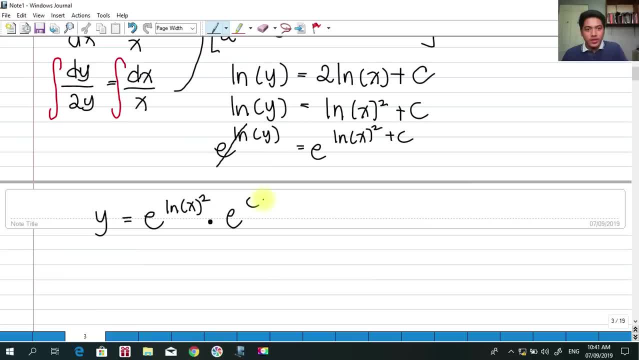 plus a mulch, multiplied by e, raised to c, because here we have an exponent. okay, that is plus. so if we can decompose this, it should be this: because we have the same base by loss of exponent: if we have the same this, the same base, we can add the exponent. so i've actually, uh, broken it into pieces. so 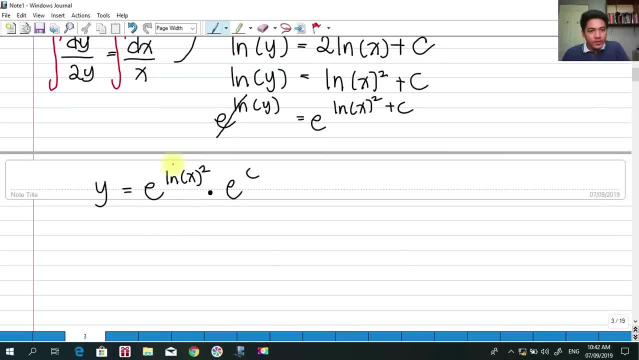 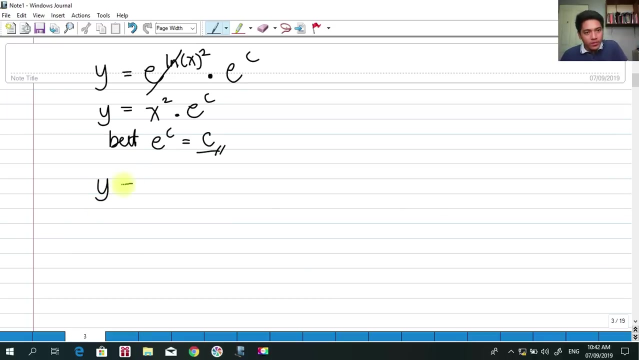 uh, for our discussion. okay, so for the sake of our discussion, we're going to cancel this again and our result will be x squared multiplied by e raised to c. but e raised to c is still simply equal to the constant itself. so in other words, we have an answer that is equivalent to. y is equals to. 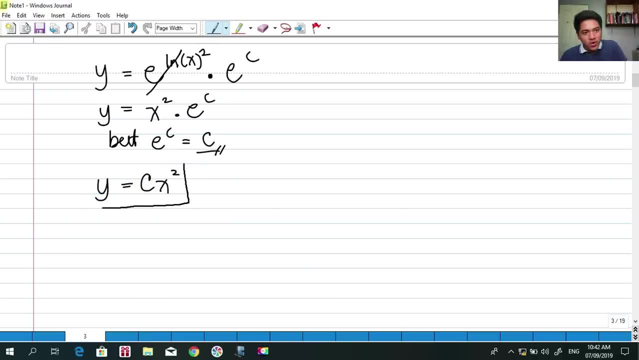 c x squared. so here we have already solved the variable separable d- e, which contains arbitrary constant c, but the constant c is not defined. so hence this is a general solution, okay, of the variable separable d- e. okay, this would be our answer. y is equal to c x squared. okay, so 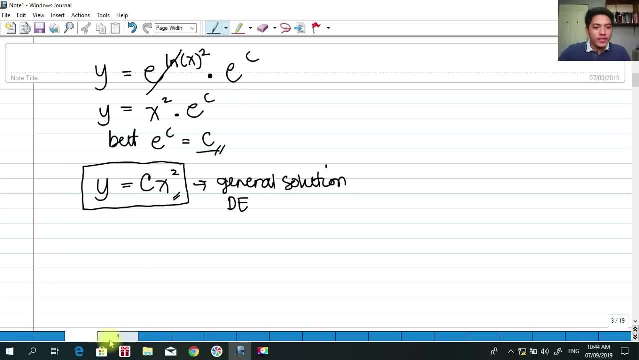 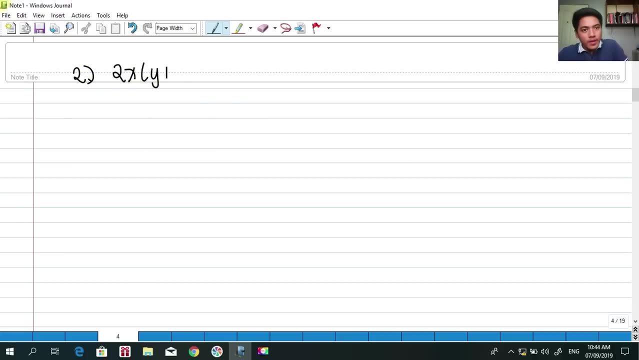 for our next example, so for number two, we have 2x times y plus 1, dx minus y. dy is equals to 0 at a given condition, at x is equals to 1 and y is equals to 0. So if we have a condition, then definitely we should be able to come up. 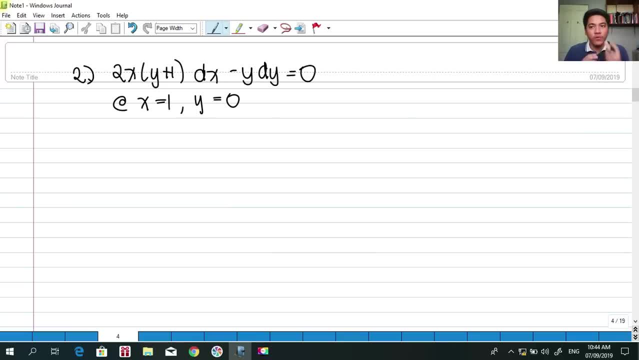 with the general solution of the DE as well, of course, the particular solution of the DE In the previous example. we don't have any conditions, so we only get the general solution of the DE. but here we have already this condition at: x is equals to 1 and y is equals to 0. definitely we can get. 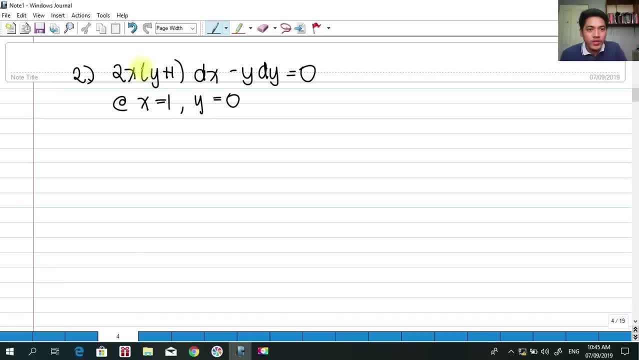 the particular solution. So, first things first, we need to separate this term okay, and group this into dy, and also, of course, what are we going to do? group first, okay, the DE's. so we have, if I'm going to multiply this or divide this, both side of the equation by 1 plus y plus 1, then 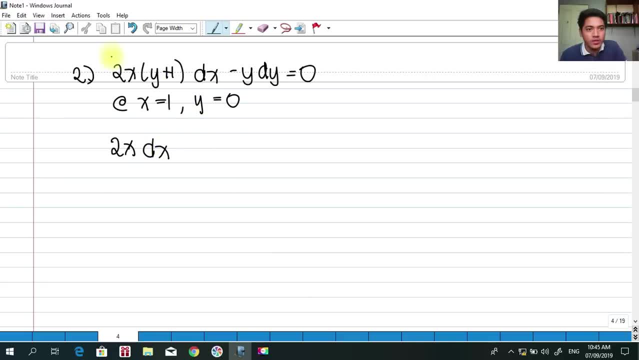 definitely this would be cancelled. this would be 2x over dx. so let me just write so that you would see: okay, so this would be cancelled. okay, and we are left with 2x dx minus. okay, y dy over, y plus 1 is equals to 0.. So here is our. we already grouped. 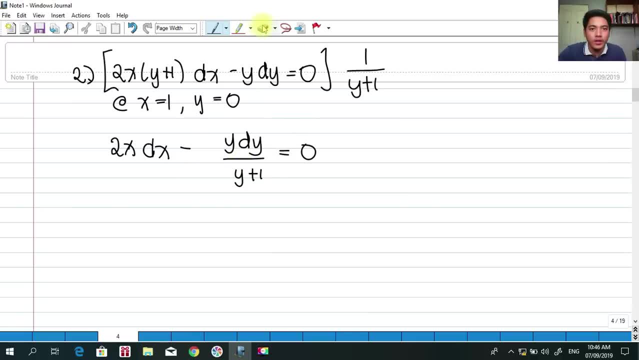 dx and all terms containing dx and all terms containing dy are now grouped with the y. so the next very step, okay, the next step is actually again to integrate. okay, so what will happen? I will just rewrite this as this: 2x dx is equals to y, dy over y plus 1. okay, if I'm going. 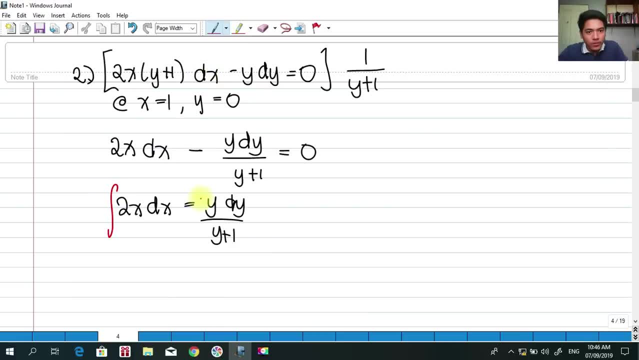 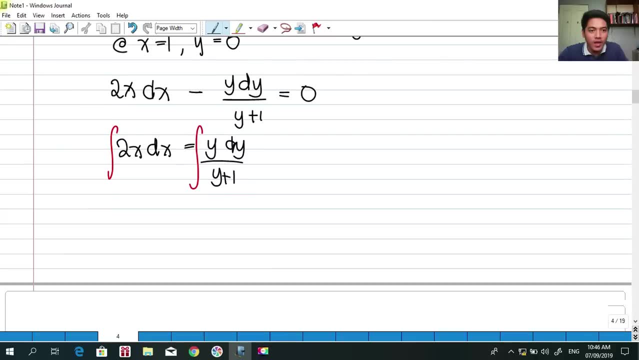 to integrate both sides of the equation, okay. so what will happen is we will be canceling the, those dx and dy, and we will be able to come up with the integration or the constant. so we have 2- the properties of integral- okay, and we have the integral of y over. 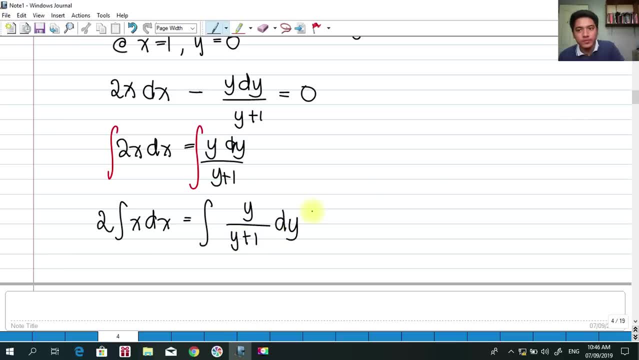 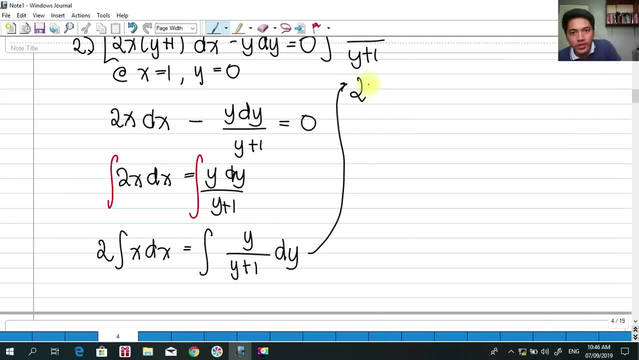 y plus 1 dy. okay, How do we integrate the left side? It's very easy. so we know that this should be x squared over 2. this would be cancelled and we are left to find the integral of y over y plus 1 dy. so we have x squared here, okay. so how do you? 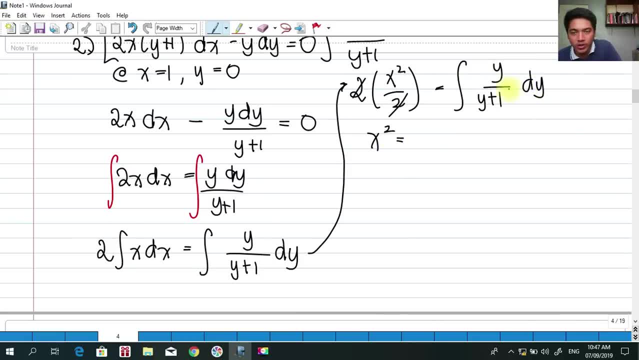 find the integral of this. okay, how do you find so? it's advisable that to find this integral, you can also use u substitution, but that is not my method. but also you can use that, but for me you can actually rewrite this integral as what we have: one i'm going to make the numerator. 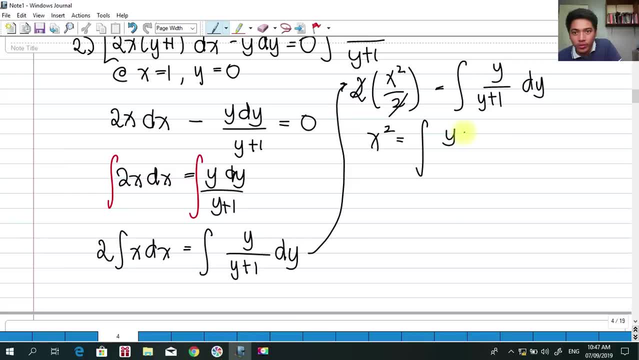 the same as the denominator. so if i'm going to add plus one also here and group it with this, and i'm going to minus one, add minus one here over y plus one dy. this numerator is still the same as y. okay, because y plus one, you can actually rewrite this integral as what we have: one. i'm going to make the numerator the. 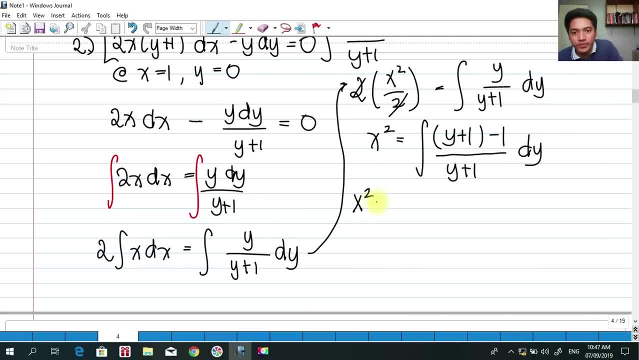 Minus 1 is still equal to y And I'm going to what Apply the rules or properties of integral. I could separate them, Okay, And evaluate their integral Okay, Such that I have this, So we have already separated this and this. 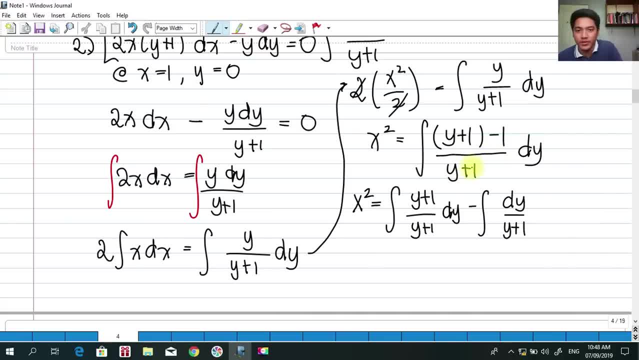 Okay, So we can only separate numerators, not denominators, Right? So this would be cancelled. So the integral of simply dy will become y, That's right, Minus, and the integral of this. Now, this is still ln, because if we make u as y plus 1,. 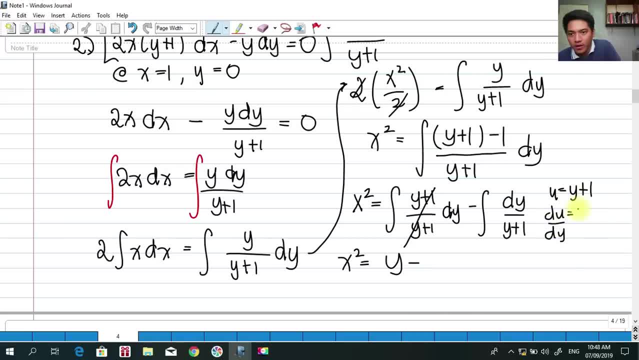 we make du with respect to dy, Okay, This would be 1.. So du is simply equal to dy. So if we're going to substitute here the u's here, So what will happen? We have dy is equal to du over. simply, u is equal to y plus 1, which is u. 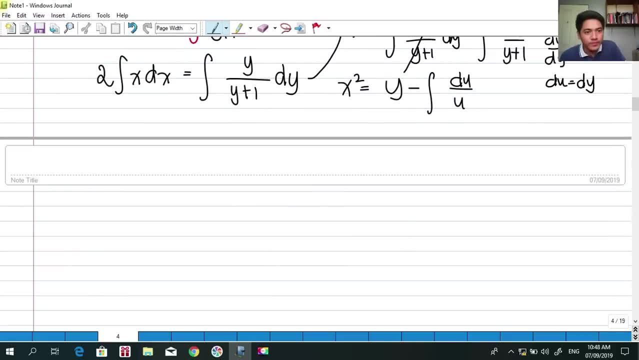 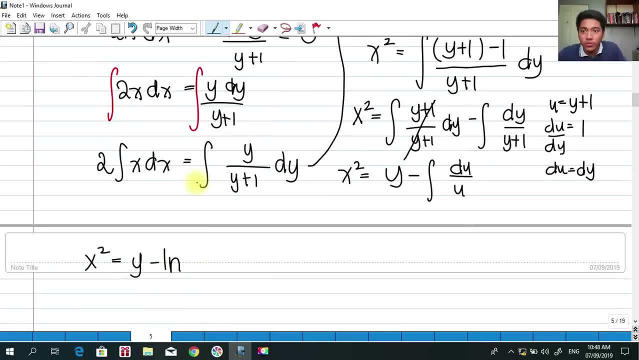 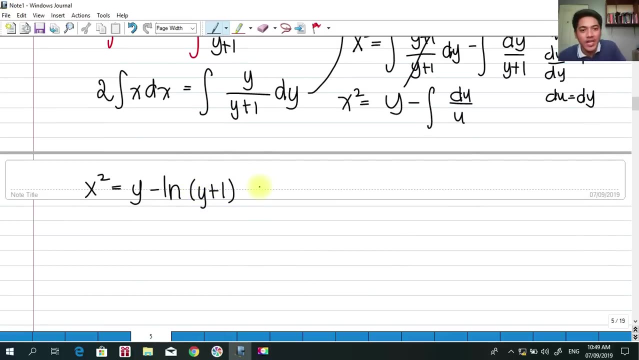 So du over u, if we get the integral of that, if we get the integral of that, simply that is yes, ln of u, Okay, But u is equal to again, u is equal to y plus 1. So we need to get it. we need to back-sub, yeah, back-substitute. 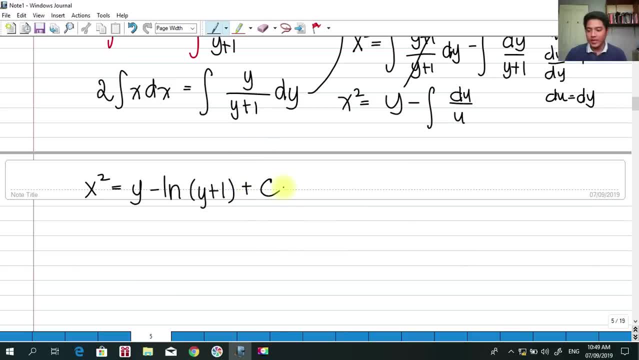 So we have upon integration, we have the constant c of course, And, as you can see, here the x does not have any natural logarithm. So, better yet, leave this. Leave this as it is Okay. We cannot cancel the ln here. 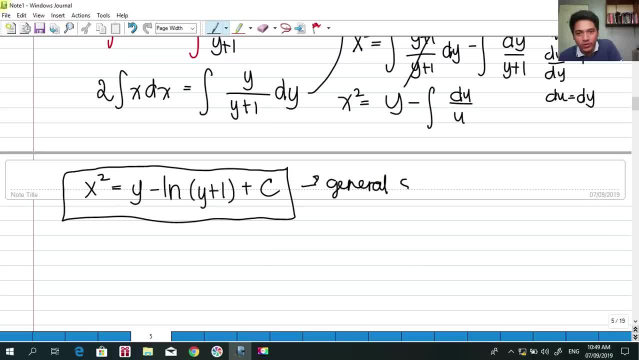 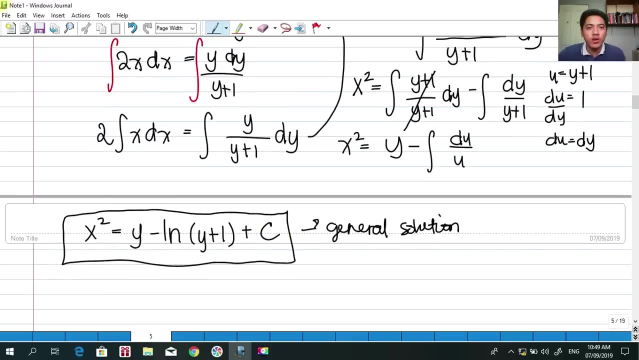 So this would be our general solution. Okay, General solution. So general solution again, a solution that contains arbitrary constant. but the arbitrary constant here is not defined. So we need to find the value of c, because we are given the equation or the condition that at x is equal to 1, y is equal to 0. 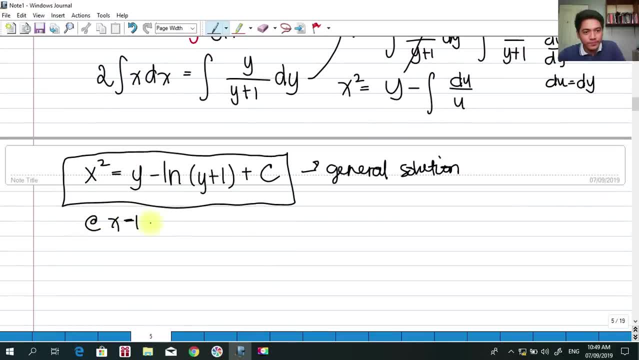 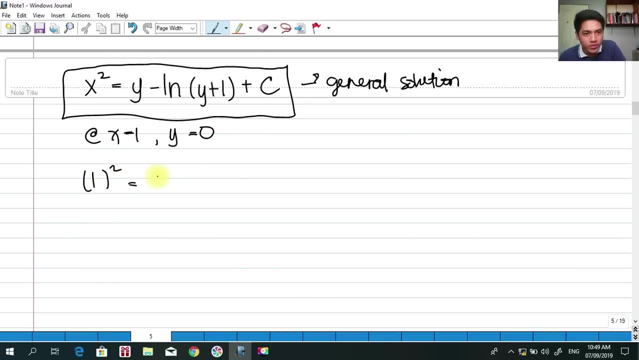 So we have the condition: c equals to 1, y is equal to 0. So what are we going to do? Simply substitute. We have 1 squared is equals to 0 minus ln of 0, y is 0, plus 1, plus c. 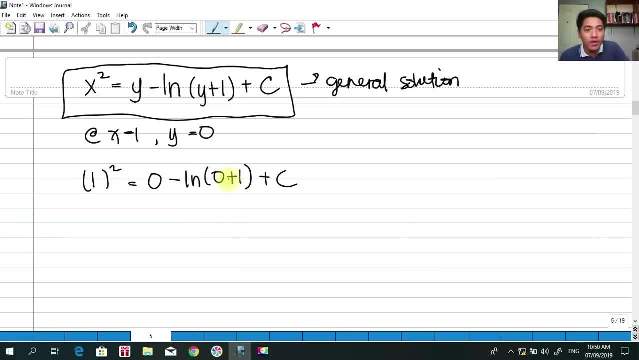 So, as you can see here, ln of 0, or ln of 1, is simply 0 also. So, in other words, 0 minus 0 plus c, then c is equals to 1, because 1 squared is equals to 1.. 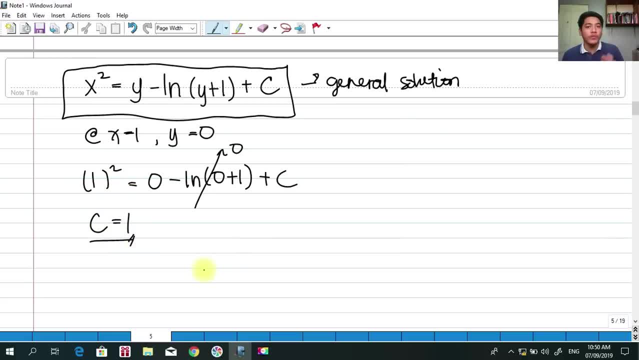 And hence, if we're going to get, And hence if we're going to get the particular solution of this differential equation, we're going to substitute the value of c to our general equation. So hence, therefore, our particular solution will now be x squared y. 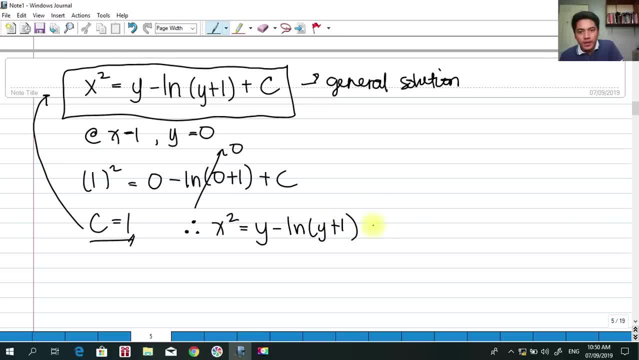 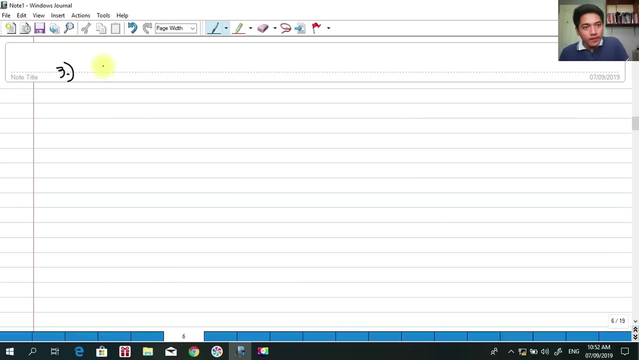 minus ln, y plus 1 plus 1,. okay, So this should be our particular solution. Hence it contains no arbitrary constant, because the constant here is defined. So this is now the particular solution. Okay, Let's solve another example. So we have for number 3, we have 2xy, y, prime is equals to: 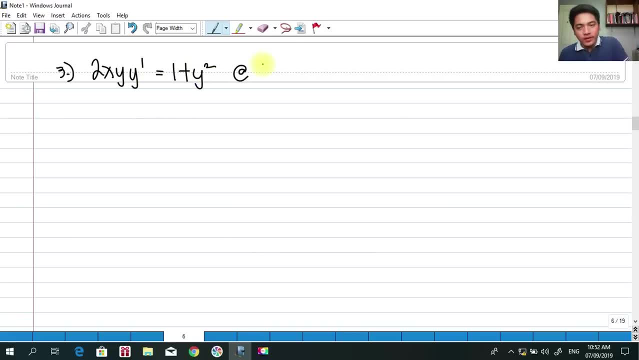 1 plus y squared At a given condition, x is equals to 2 minus 1 plus 1.. So we have 2xy. y prime is equals to 1 plus y, squared At a given condition. x is equals to 2 minus 1.. So we have 2xy. y prime is equals to 1 plus y, squared At a given condition. 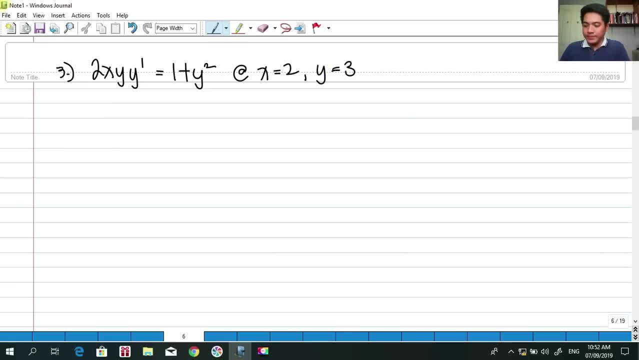 y is equals to 3.. Okay, So first things first, we need to group them in terms of dy and dx. So we have 2xy. y prime is equal to simply dy over. dx is equals to 1 plus y squared, And if we cross, 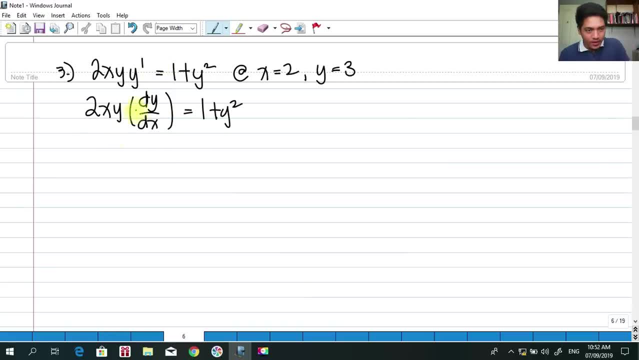 multiply dx to the both sides of our equation, so we have 2xy. dy is equals to 1 plus y squared. We have dx here And we need dy here. We need all terms of y to be in here and all terms of x to be. 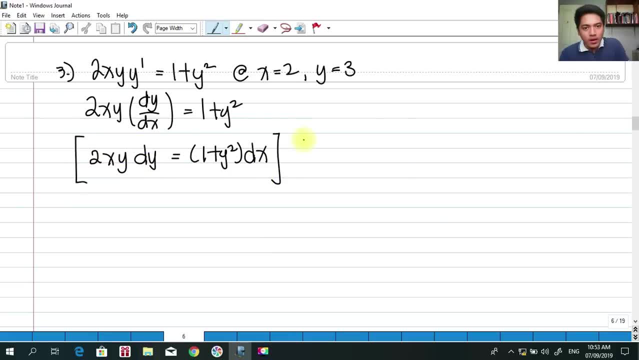 in here. So hence, if I'm going to divide them both sides by, let's say, I would like to divide it by, let's say, 2x, because I want to cancel 2x here And I need to have 1 plus y squared here. So I 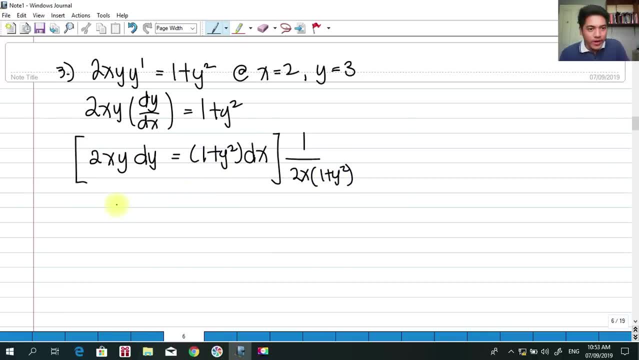 would like to cancel 2x here And I need to have 1 plus y squared here. So I would like to cancel here, cancel this here. So what will happen? we have an equation that is y dy over 1 plus y squared. 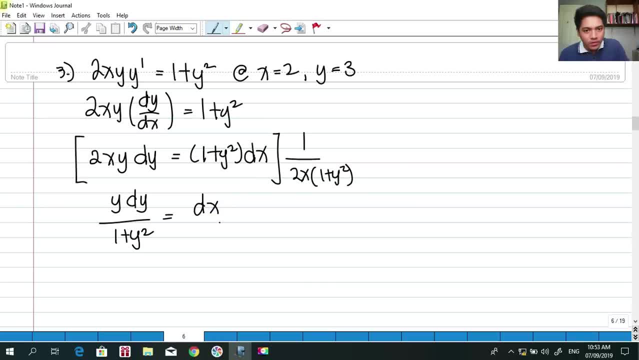 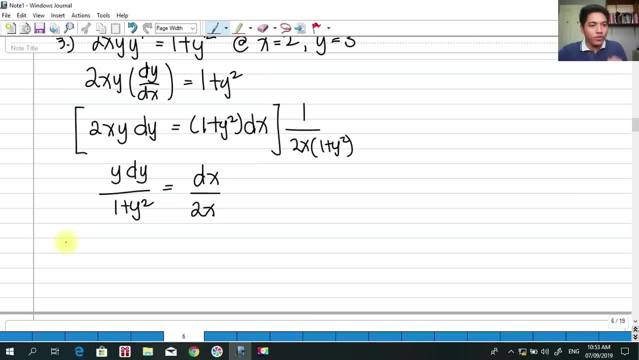 is equals to: we have dx over 2x. Okay, So hence we group all terms of y in dy, all groups of x in dx. So the next step again is to integrate both sides of our equation and upon integrating we shall arrive or we shall eliminate the dy and dx here. So we have here: 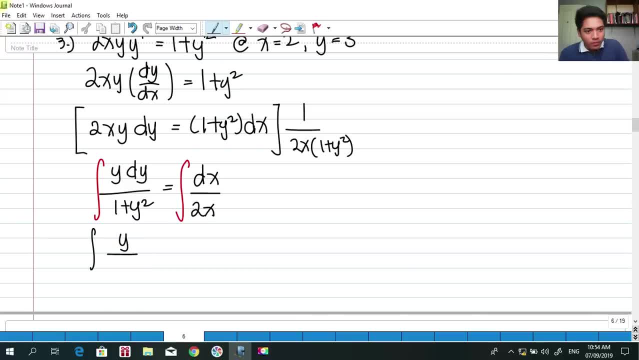 okay, integral of. let me just rewrite y squared plus 1,, okay, dy, And we can factor out one half outside of the integral sign again, so that this is dx over x. Okay, So how do we integrate this? 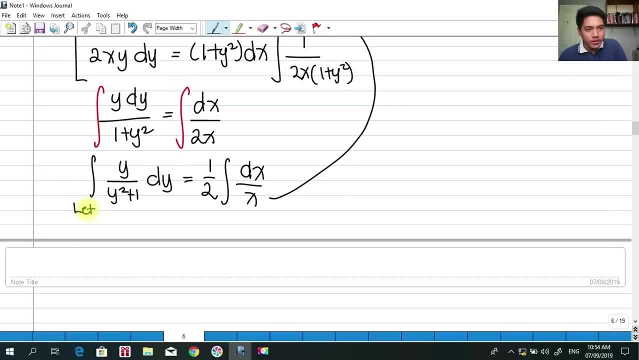 So here we can use the u-satisfaction If we left u as y squared plus 1, and du with respect to y is 2y dy. So I have an available here of y dy. This is my y dy, Okay, But I have to offset 2 here because the du is actually 2y dy. 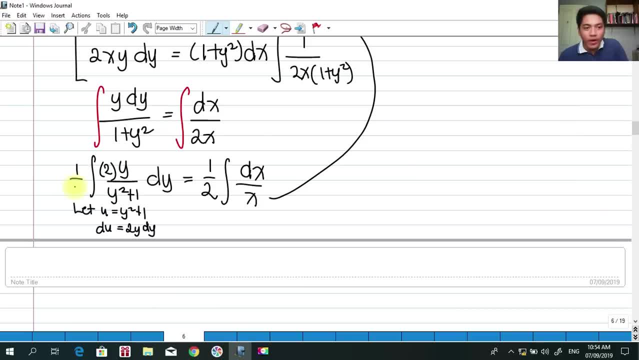 but I have also have to correct it by a correction factor outside of the integral one half. So whatever it is that you multiplied inside of the integral just to satisfy this du, you're going to get the reciprocal of that And again add it or multiply it outside of the 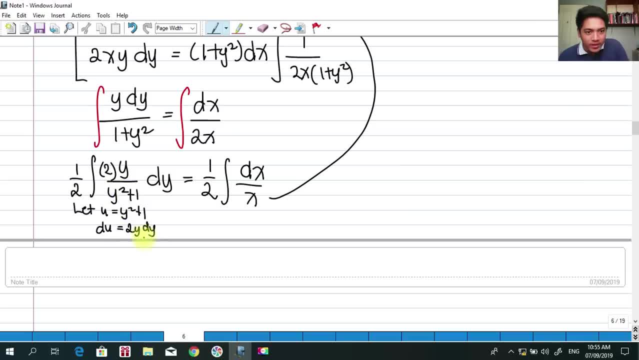 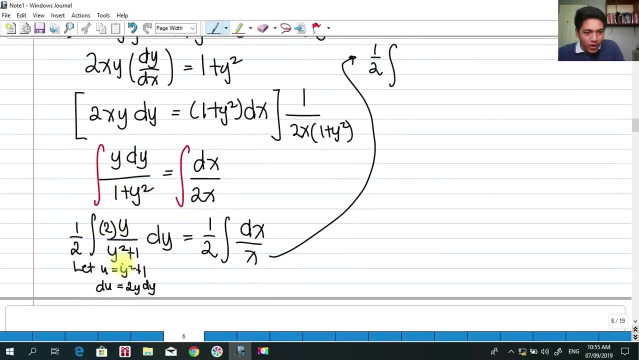 integral. So in this case we added 2 to satisfy this, to perform u-substitution, And the reciprocal of this is one half. So you're going to multiply it one half. That is the correction factor, So that I would be able now to write this as the integral of 2y dy. 2y dy here is simply equal to. 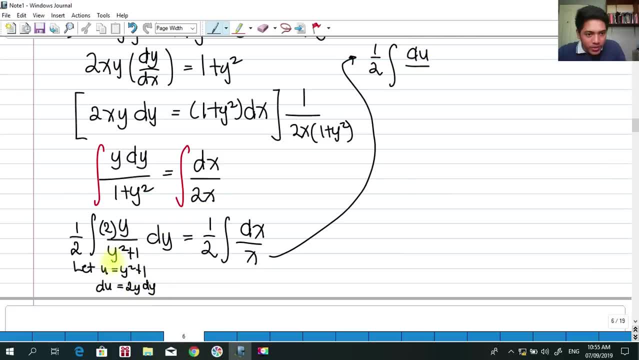 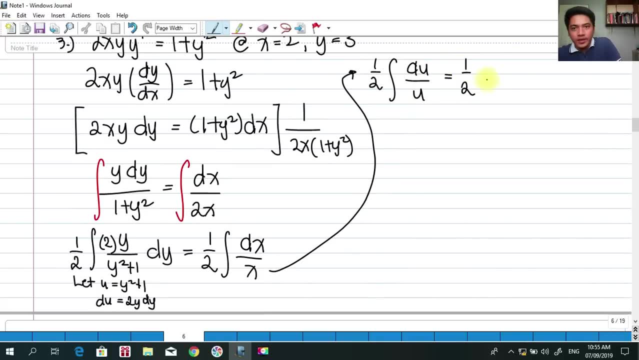 du over what is our u, y squared plus 1 is u So over u, And again, equal to one half dx integral of dx over x. So this is both our logarithm. So we have one half ln of u, okay is equal to one half ln of x plus c. 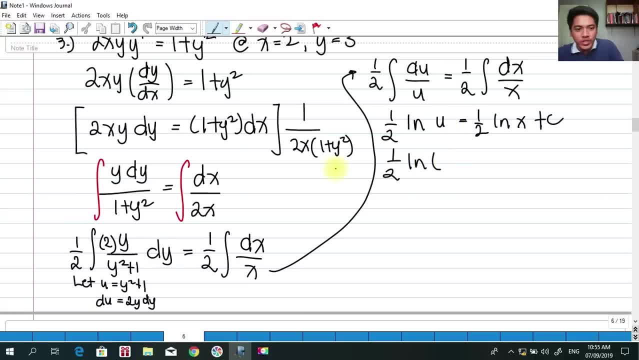 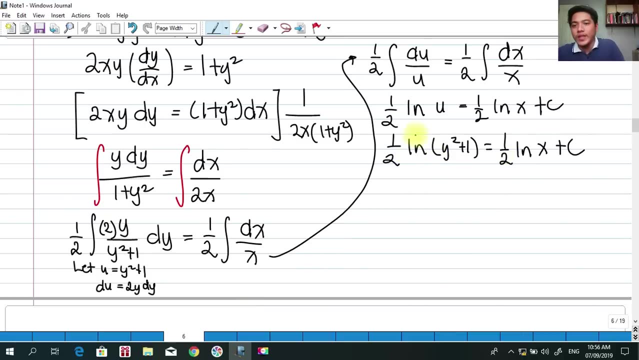 But we need to substitute back u to its original substitution. So we have ln of y squared plus 1, because u is equal to y squared plus 1.. As you can see, both of the x and the y contains ln, So we can multiply both sides by 2 so that we 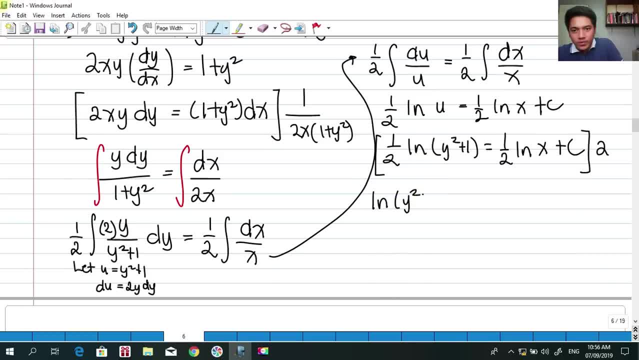 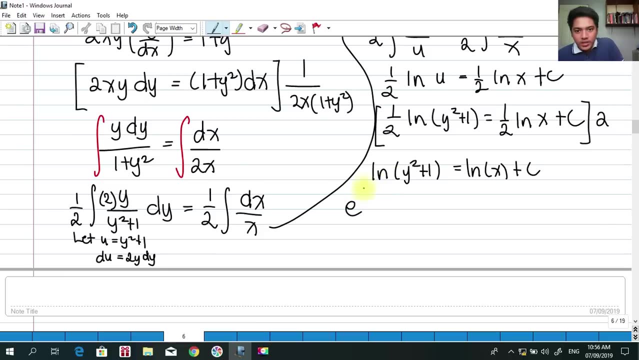 can eliminate one half here, So that we have ln. y squared plus 1 is equal now to ln of x plus c. That should be our result, And in order for us to eliminate the ln again we did a while ago, is we need to raise this both side of the equation with e, So y squared plus 1. 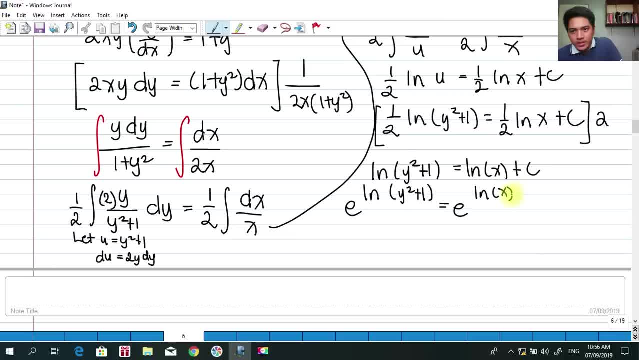 is equal to e ln of x plus c. So this should be cancelled, okay, And whatever left inside of the ln. that should be our result. y squared plus 1 is equal now to by laws of exponent. again, I can decompose it into this: okay, Because of law by law of exponent. 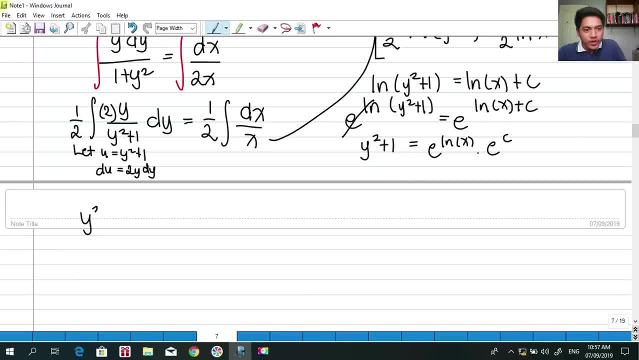 is equal to this. okay. So what will happen? y squared plus 1 is equal now to. this should be cancelled. So simply x multiplied by e, raised to c. okay, And again e raised to c. this term is simply equal to. 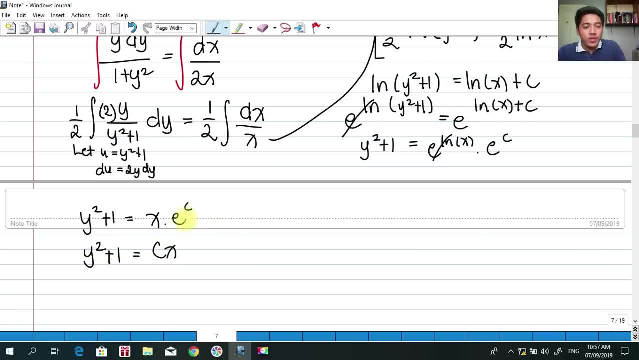 that's correct. simply equal to c. simply equal to c multiplied by x. So this should be our what We have: an arbitrary constant of c, So this should be our general solution. General solution. okay, Let me just rewrite. So we have: 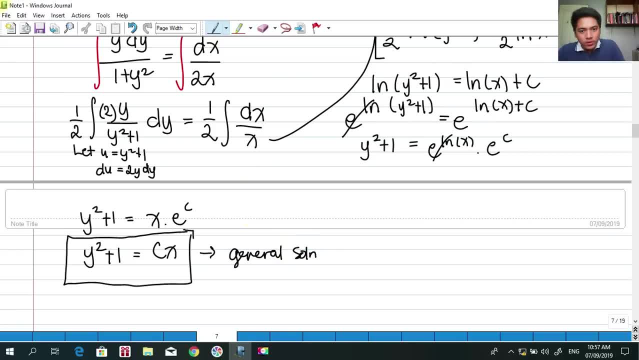 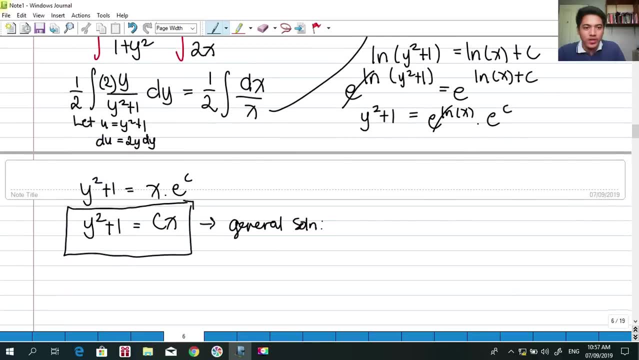 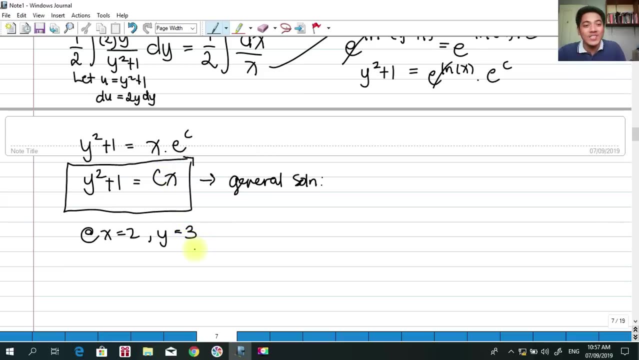 the general solution. okay, But we have a condition. A condition is x at x is equal to 2 and y is equal to 3.. So definitely we need to find the value of the c in order for us to satisfy the condition. 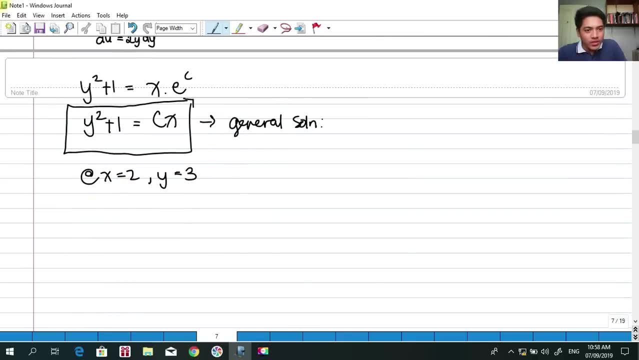 That's a particular solution. So at x is equal to 2, that is, 2 squared plus 1 is equals to. I mean, that is not 2, that is simply 3, because our value of y here is 3.. So 3 squared plus 1 is equal to c times 2,. 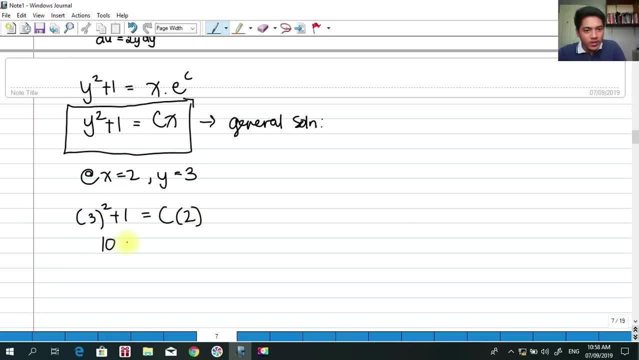 okay, So this is 10.. 3 squared is 9 plus 1, 10.. We have 2c here, So c is therefore 5.. So, again to get the particular solution, simply substitute the value of c on our value of y. So, again to get the particular solution, simply substitute the value of c on our value of y. 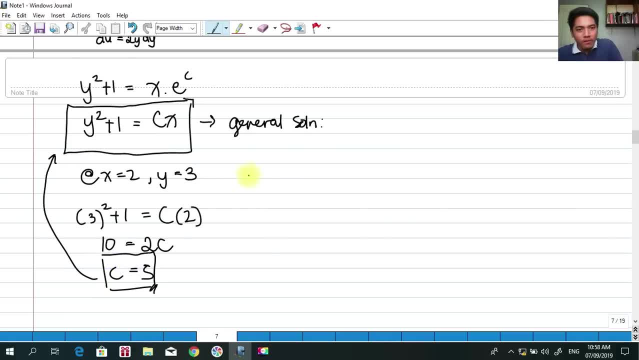 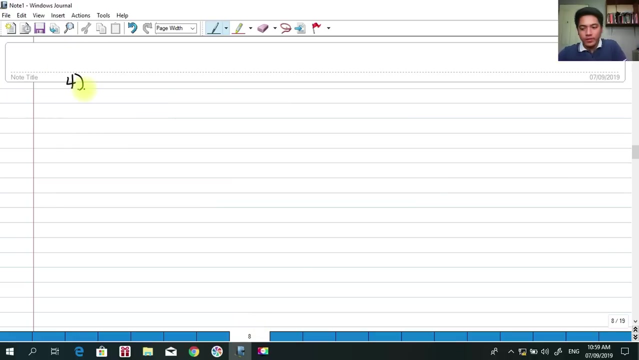 So this should be our general solution. okay, So we have y squared plus 1 is equal now to 5x, So this should be our particular solution. Okay, so for another example. so we have number 4.. We have x cubed plus 2.. 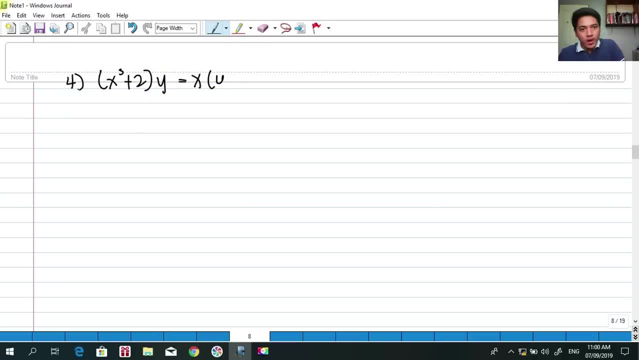 We have: y is equal to x, y raised to 4 plus 3, y prime at a given condition: that x is equal to 1 and y is equal to 1.. So again, same first step We need to express all of. we need to group dx and dy with x and y respectively. 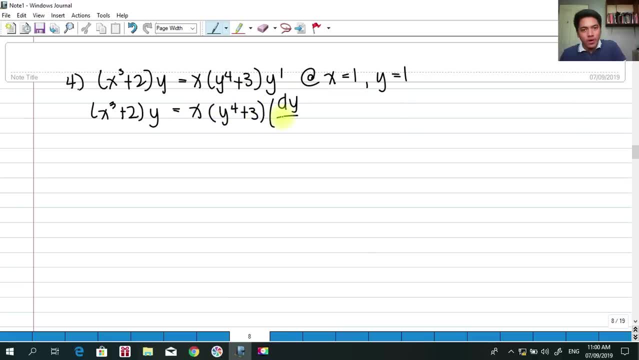 So we have this: y prime is simply equal to dy over dx. So I'm going to do this: Multiplying both sides of the equation by dx, we have x cubed plus 2, y. dx is equal to x. y raised to 4 plus 3, dy. 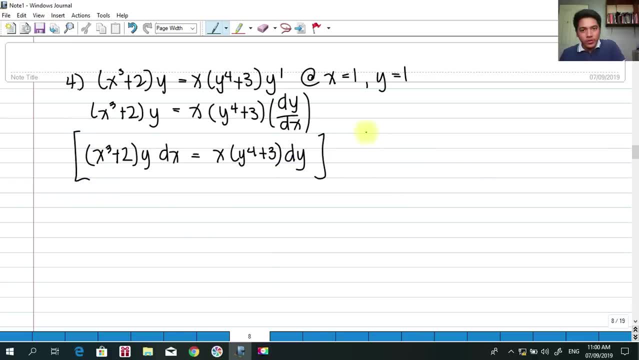 And if I'm going to divide the whole side of our equation by y- y because of this, we need to eliminate this. And here with x, y over x. so simply, what will happen is we have x cubed plus 2 over x dx. 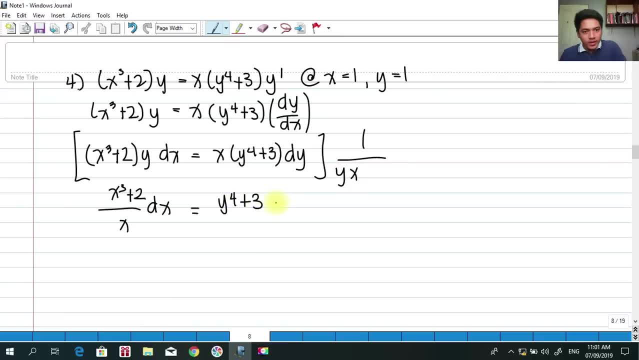 is now equal to y, raised to 4, 3 dy okay, over y, and upon grouping them. the very next step is again, integrate both sides of our equation so that we need to have or we can eliminate x and dy. 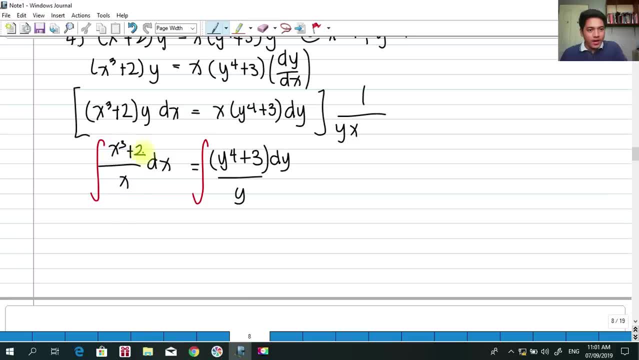 So, upon integrating this integral can be simplified as we have x cubed over x dx, x cubed over x dx, x cubed over x dx, Always distribute the integral sign. if we have some or minus here, Okay, and the dx, of course, plus 2.. 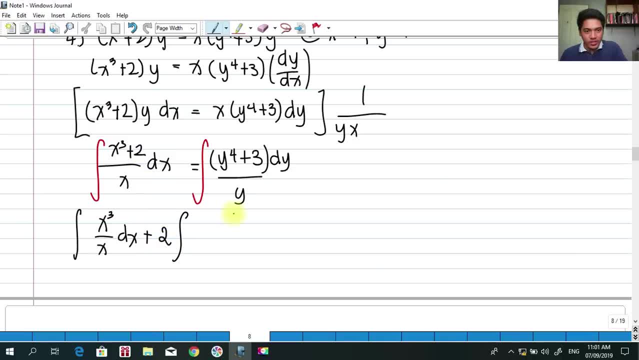 I'm going to bring this outside of the integral because it's constant. So we are left with dx over x And that is equal to the same process: y raised to 4 over y, plus bringing out 3 here because it's constant. 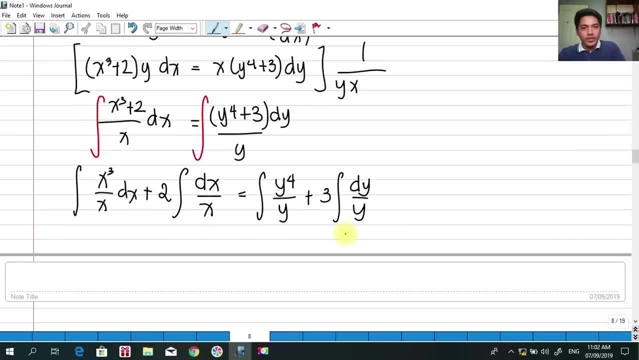 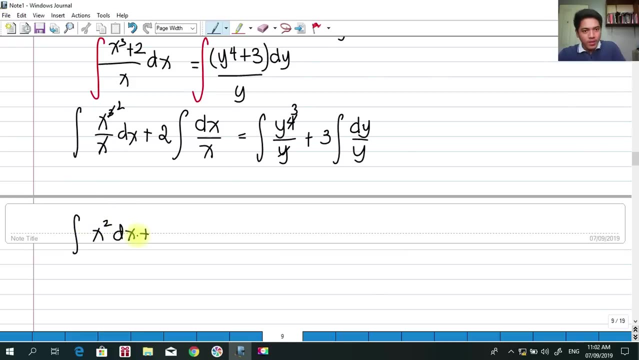 So we have dy over y And we can simplify this by: this should cancel: This should be x squared. This should cancel: This should be y cubed. And proceeding to our integral, now we have the integral of x squared dx plus 2. integral of dx over x. integral of y cubed plus 3. integral of dy over y. 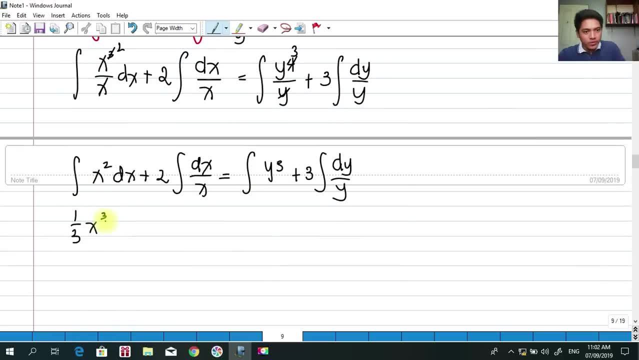 So integral of x squared dx, that is 1 third x cubed plus this is ln. again, 2ln of x is equal to 1. fourth y raised to 4. integral of y cubed plus 3ln of y. forget the plus c. 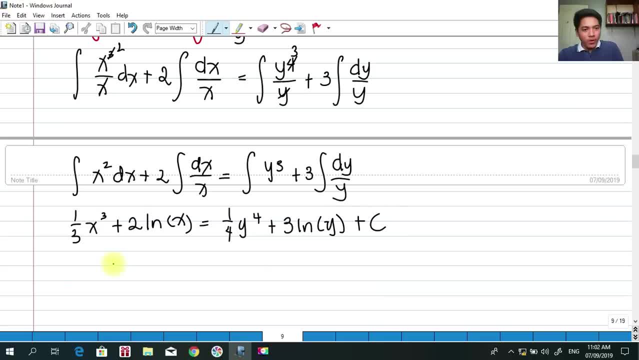 Okay again, since both here we have an x term that is in terms of logarithm and we have an x term that is not in logarithm. okay, we cannot cancel out. Okay, We can easily do ln. okay, here the same here. 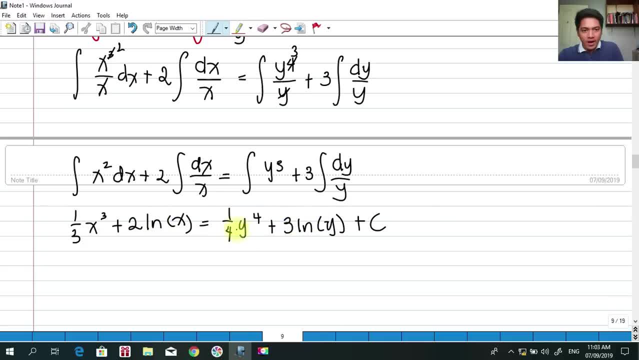 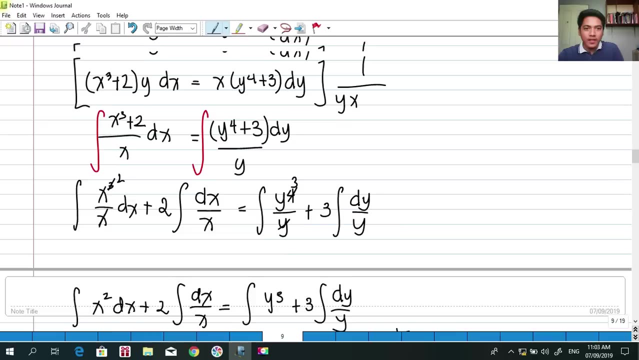 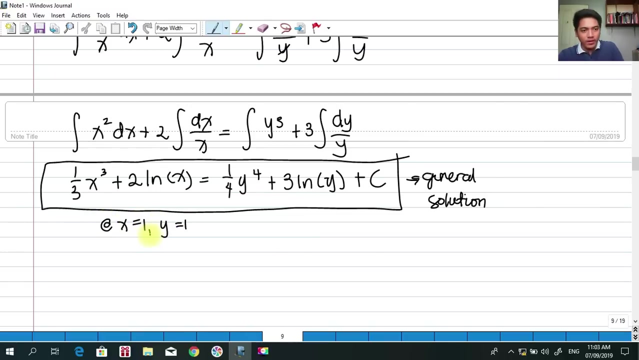 We have 3lny and the other one is in this form, So we cannot cancel, So we can leave it as it is. So, therefore, this is our what general solution, But take note that we have a condition, And that condition is that x is equal to 1, okay- and y is equal to 1.. 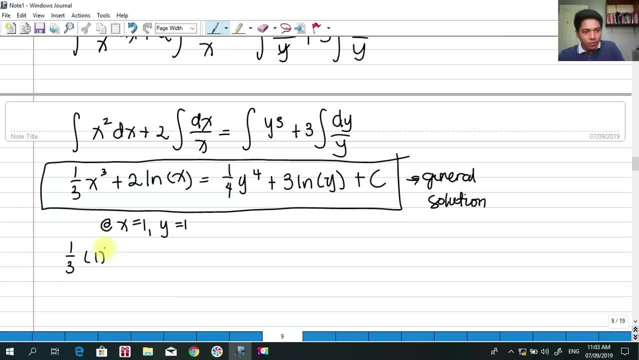 So we simply substitute the values: 1. third, 1 cube plus 2ln of 1.. This is 0, simply 0, because ln of 1 is 0. It's equal to 1. fourth, 1 raised to 4 plus 3ln of 1.. 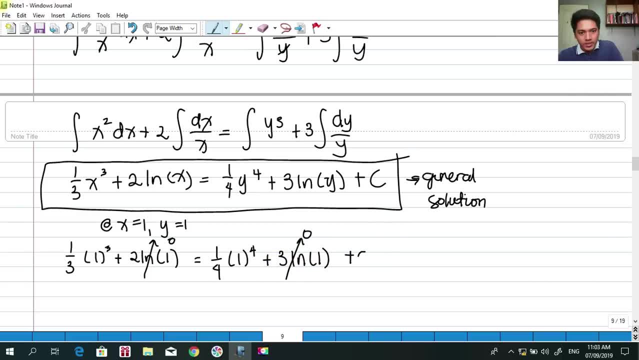 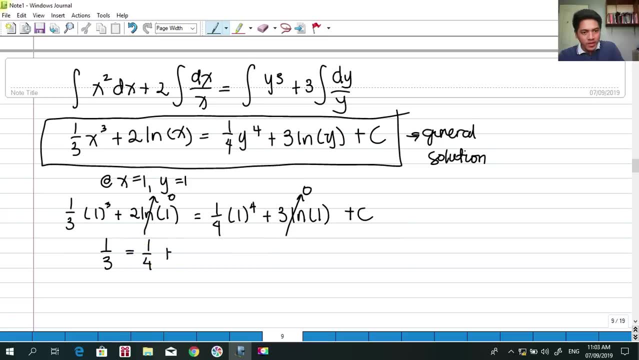 This is simply 0, ln of 1 is 0, plus c. So, as you can see, 1 cube is still 1, 1 raised to 4 is still 1.. 1 third is equal to 1 fourth plus c. 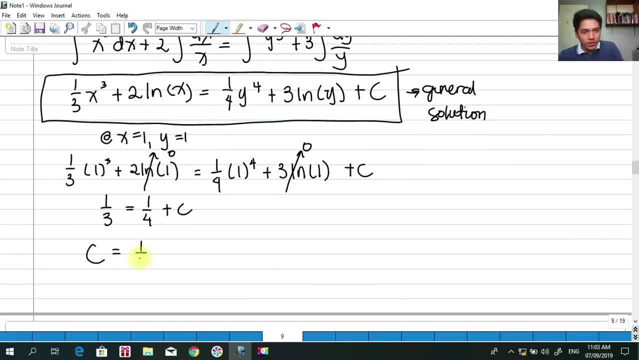 We need to find c. c, therefore, is So 1 third minus 1 fourth. Okay, so what will happen here? 4 minus 3 over 12 is 1 over 12.. So our value of c is 1 over 12.. 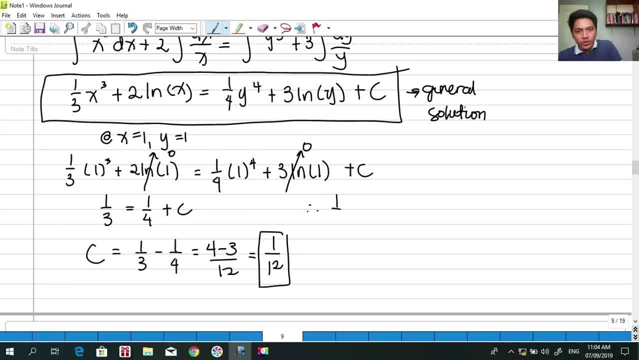 Hence, therefore, our solution, or particular solution, will be: 1 third x cube plus 2ln of x equals to 1 fourth y raised to 4 plus 3lny, Why Plus 1 over 12.. So this is our particular solution for this problem, okay. 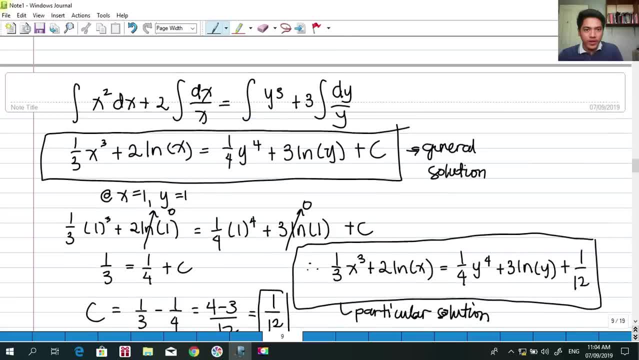 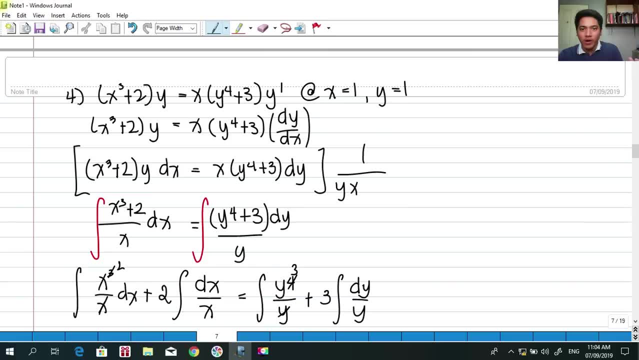 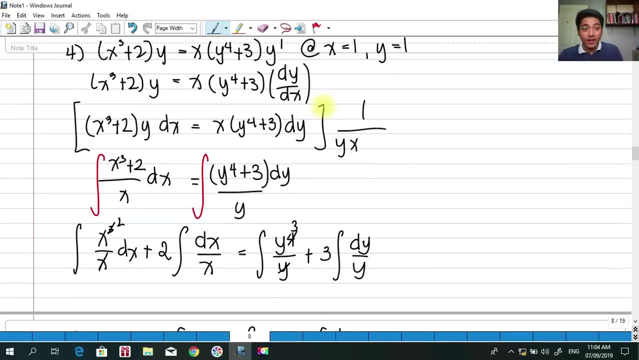 So, as you can see, differential equation, solving differential equation: okay, first we need to group in terms of d, y and d x. That's when the differential equation part is done. okay, The next step is to integrate Again integral calculus. 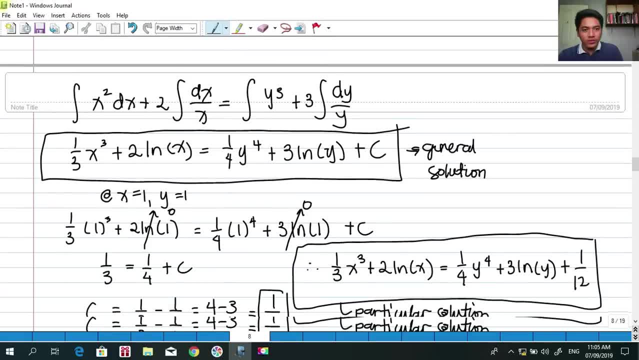 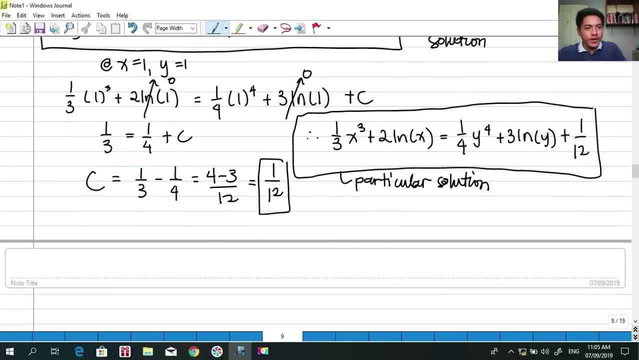 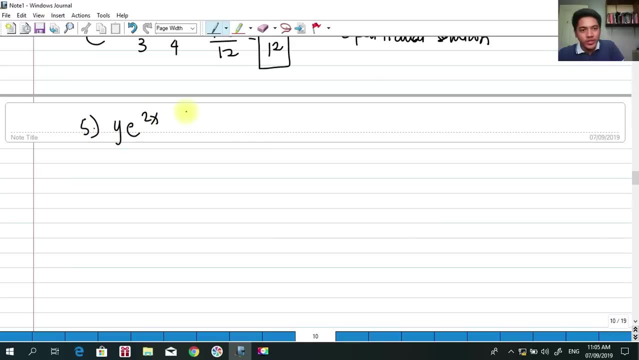 It's essential. And after integration, algebra part is essential also. okay, Okay. so next problem: you know, the only way for you to be good or to master your mathematics subjects is none other than solving many problems, as again So in this video, I always give many examples for the viewers to really practice. 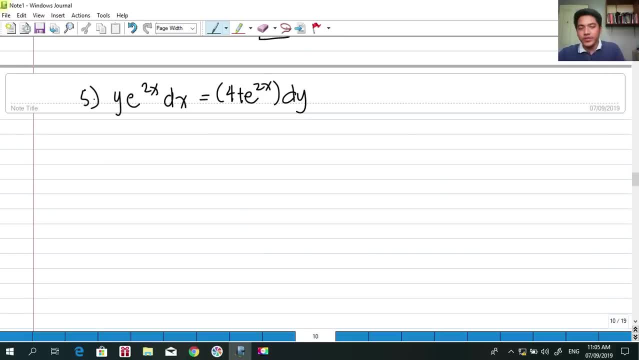 So there's no other way for you to be good at math rather than solving many, many problems. All right, here. this is a variable separable d, e, and we can simply what separate it: e raised to 2x, d, x, by simply multiplying or dividing both sides of the equation by 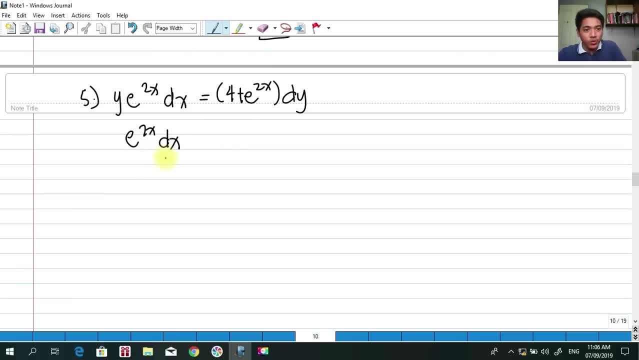 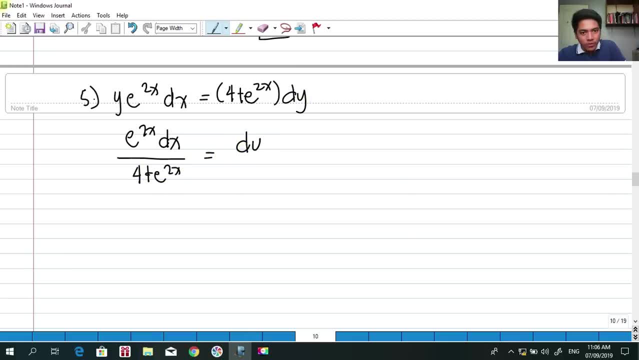 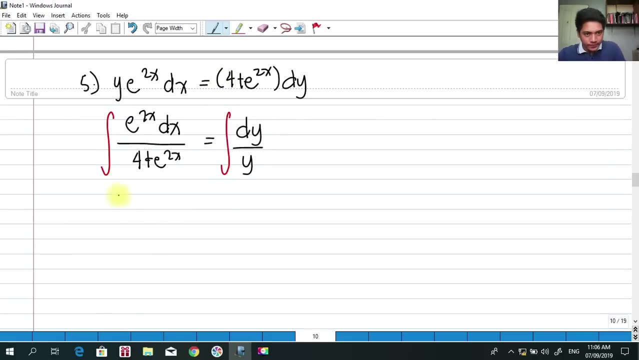 So that we have 4 plus e, raised to 2x here, and we have, of course, dy over y here. So again, upon grouping them, we need to integrate both sides of our equation for us to find the constant okay or the general solution. 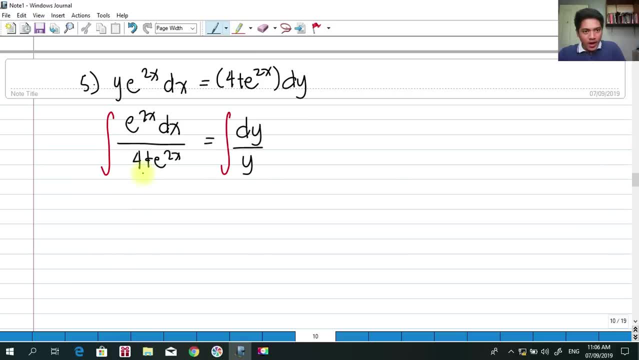 So how do we integrate this? As you can see here, this integration involves u substitution. Why? Because this: if we let that as u, Okay, 4 plus e, raised to 2x, if you get the derivative of u with respect to x, that is. 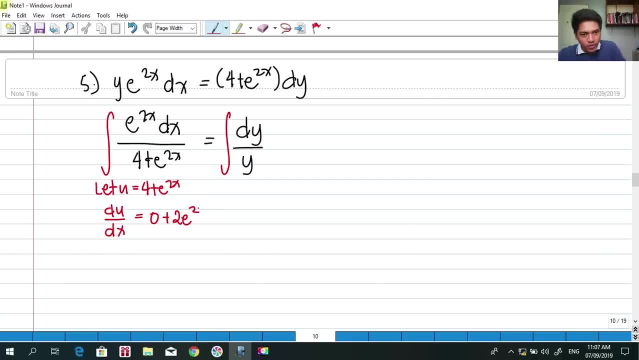 simply 0 plus 2e raised to 2x cross-multiplying the dx. here we have. du is equal to 2e raised to 2x dx and e raised to 2x dx. is this okay? 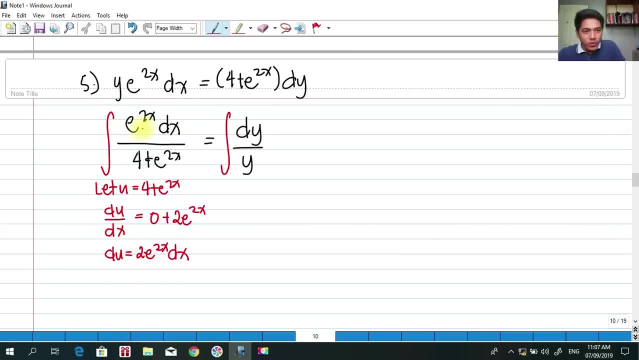 But again, our upon differentiating, we have 2 here, so we have to offset 2 here. Offsetting 2 here, we should offset outside of the integral 1 half for our correction factor, And hence we can now perform the u substitution. 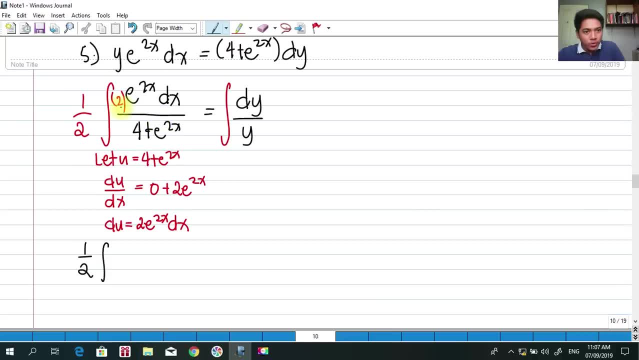 So we have 1 half integral of 2e raised to 2x. 2 times e raised to 2x, dx is simply equal to du over 4 plus e raised to 2x, that is simply du okay. 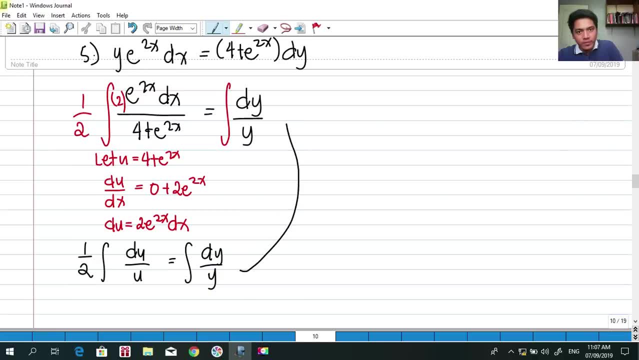 Integral of dy over what? So this is pretty much easy. So this is still ln. ln of u, Okay, Is equals to dy. integral of this is ln of simply y plus c, Don't forget d plus c, okay. And of course we need to back substitute u, as this: 4 plus e, raised to 2x, is equals. 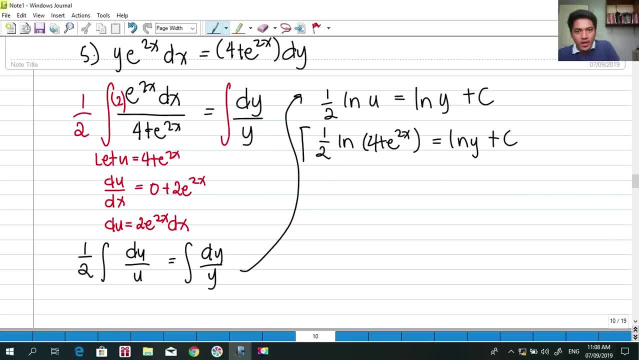 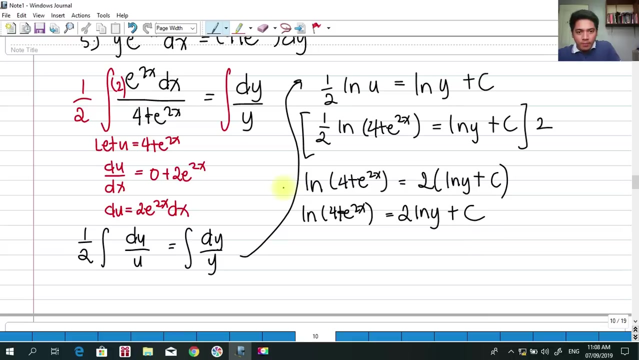 to ln of y plus c. We can multiply both sides of the equation by 2 to eliminate 1 half here. so we have ln 4 plus e. raised to 2x is equal to twice the ln of y plus c. So we have ln 4 plus e raised to 2x is equal to 2 ln of y plus 2 times e, still c. 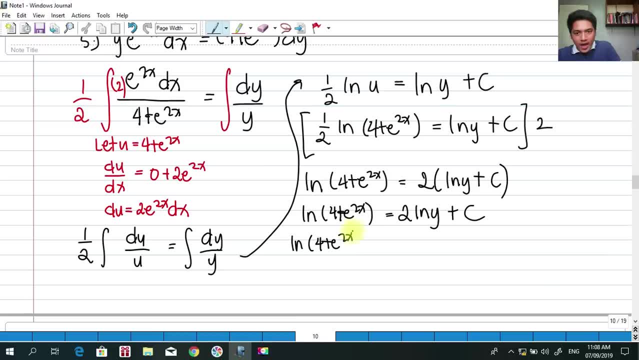 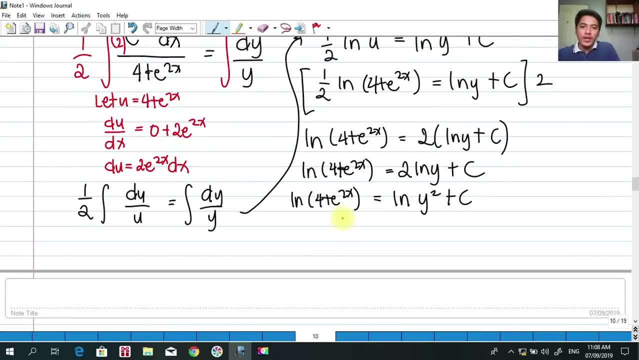 By properties of logarithm we can have, we can rewrite this: 2 ln, y as ln of y squared plus c. Okay, In order for us to eliminate ln- because we have ln in terms of x, ln in terms of y- we 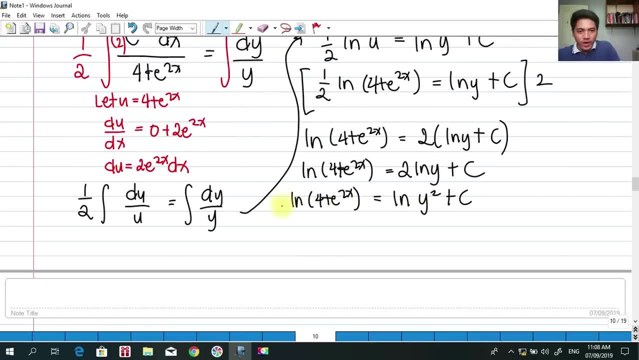 can write this: 2 ln y as ln of y squared plus c. Okay, In terms of x, ln in terms of y. we can again raise them up. okay, by by e. So we have ln of y squared plus c. 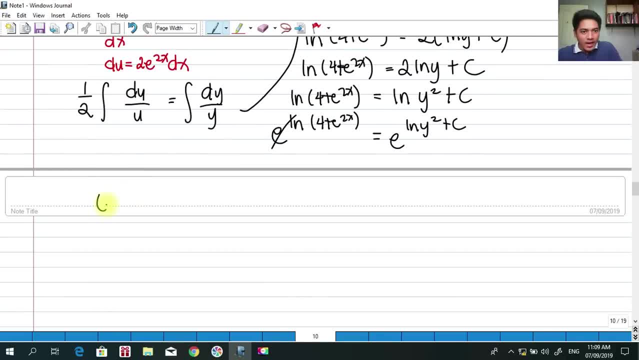 So this should be cancelled. So whatever left is the answer for that. 4 plus e raised to 2x is equals to: this can be written as this side can be written as by loss of exponent again as this: So we have 4 plus e raised to 2x cancelled. 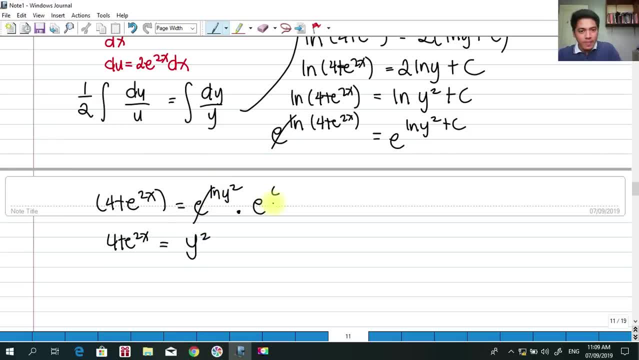 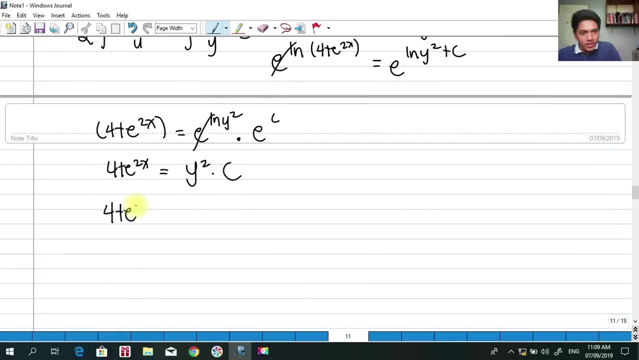 So we have 4 plus e raised to 2x cancelled, So we have y squared. e raised to c is simply equal to c, So we have an answer that is: 4 plus e raised to 2x is equals to cy squared okay. 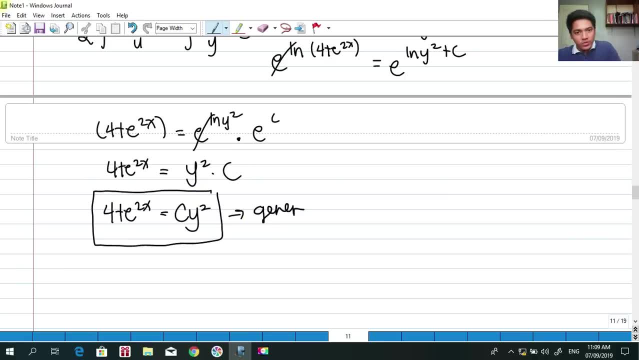 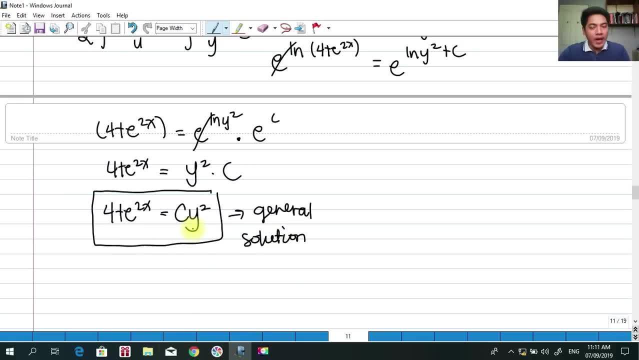 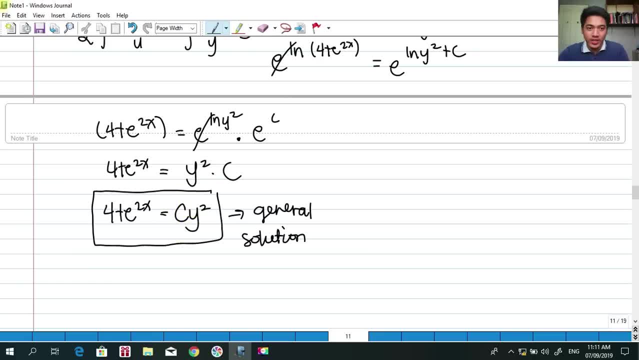 c is raised to square q, sometimes to c, But I haven't seen like that before. So if we encountered c squared here instead of c, that is still correct answer. That is still a correct answer. okay, The c here is actually what. 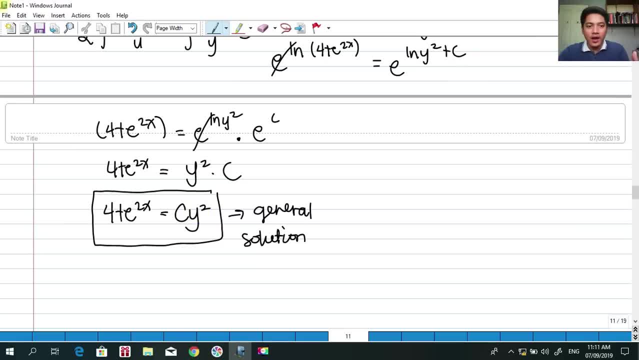 The c squared. it doesn't matter where this c is raised to, Oh or twice a number, it is still C at the end of the day. okay, so if you see an answer of C squared, Y squared in this for this example, okay, because if we 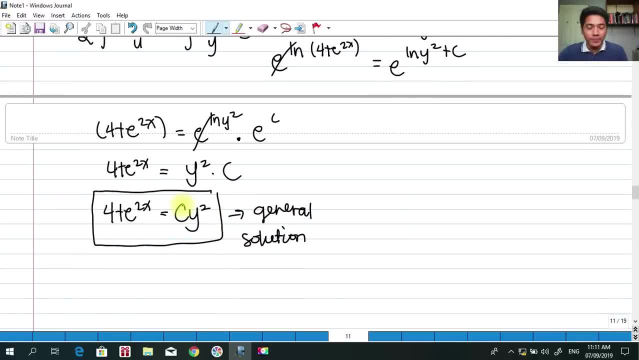 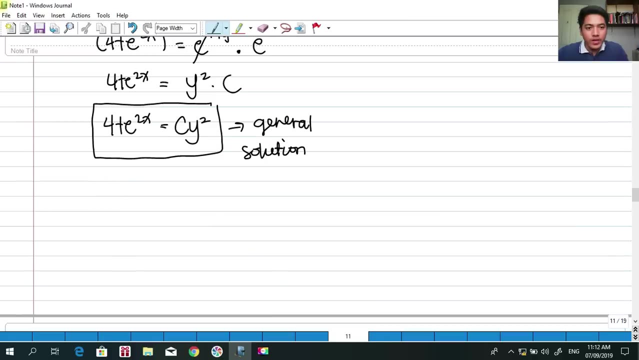 solve it in another way, we will be ending up with C squared. okay so, but still, that C squared is equal to a constant C. okay, let's try to solve another problem. okay, so, let's try. let's try this number six we have MY DX- is equals to NX DY. so, as you can see, here, M and N are actually constants because we 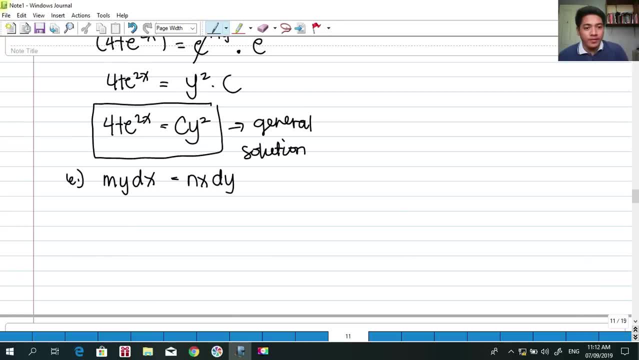 are concerned with integrating the in terms of DX and DY, so any variables rather than X and Y are considered as constant. so in this case, so we can what we have: M, DX, we need to get X. so over X is equals to N, DY, over, we need to get Y here. so this would be our equation if we 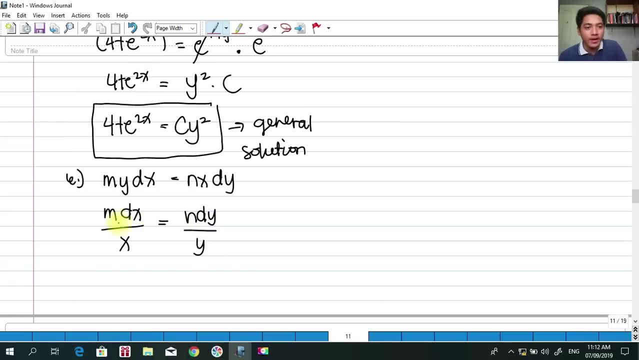 group them in terms of X and in terms of Y. note that M and N are constant, so we have to integrate both sides of our equation and then, upon integration, we can rewrite this as M, DX over X. because M is constant, we can move it outside of the integral sign and N. 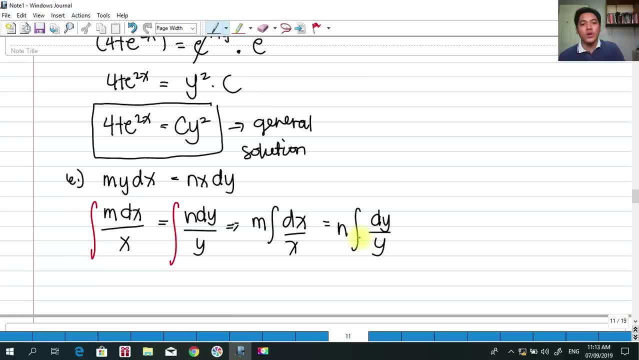 integral of DY over Y, so that we can integrate now: M LN of X equals to N LN, natural logarithm of Y plus C and by properties of natural logarithm this can be written as: LN of X raised to M- okay is- equals to LN of Y raised to N plus C. upon. 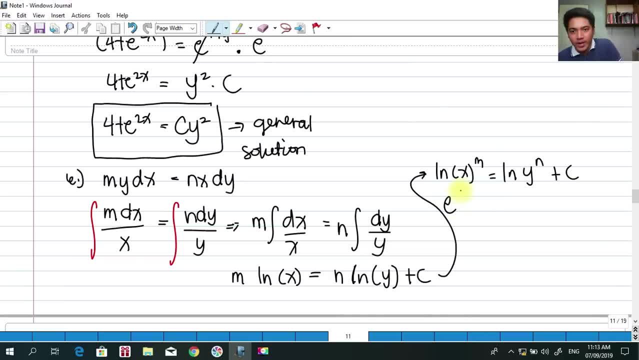 eliminating again the LN. we need to raise them as LN X raised to M is equals to E- natural logarithm- Y raised to N plus C, and of course this should be X raised to M, and we know what will happen to this. so E LN Y raised to N times E raised to C by: 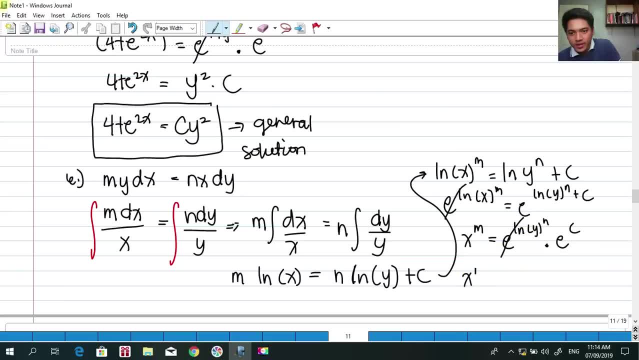 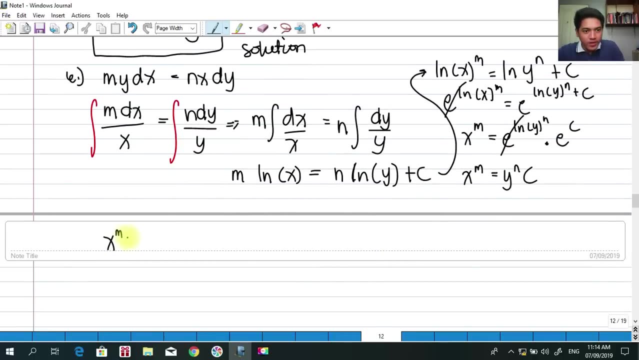 properties of exponent, and again this should be canceled. the X raised to M- okay, is equal now, is equal now to Y raised to N: okay, C multiplied by C. or, in other words, to look it nicer for you to look it nicer that your answer- X raised to M. 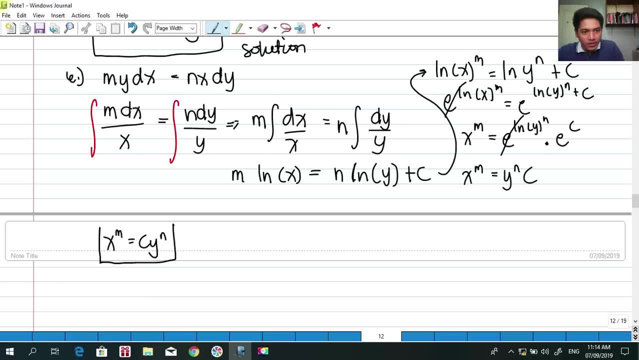 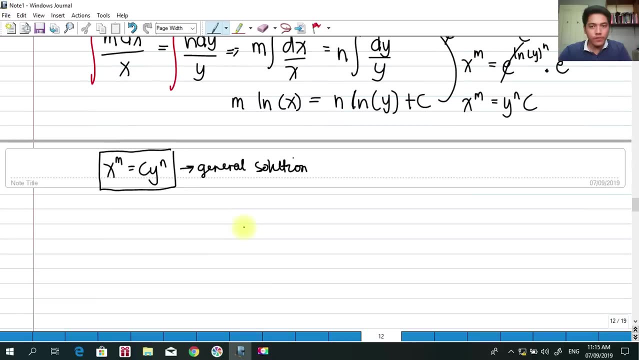 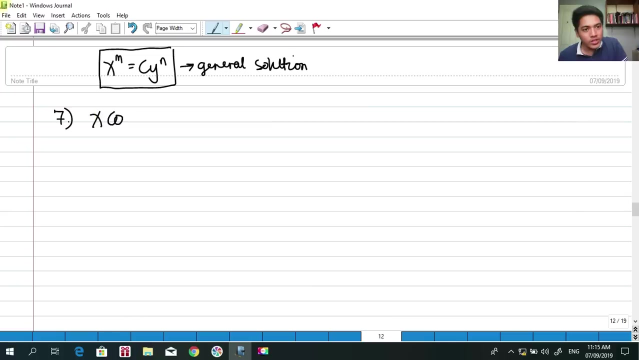 is equal to C Y raised to N, and so that should be our general solution, since we don't have any condition set in our problem. okay, so for number seven, let's let's try to look at this number seven: X, a cosine squared Y, DX plus tangent of Y, dy is equals to zero. okay, so we still. 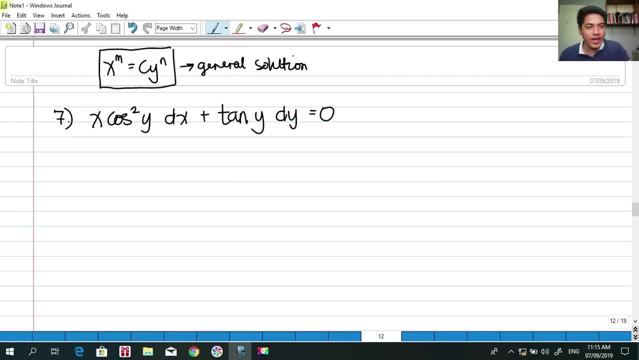 we need to group them in terms of X or DX, Y or dy. so, as you can see here- this is the problem- cosine squared of Y. so we need to get it here. so we have what we can multiply or divide both sides of the equation by one cosine squared of Y. so 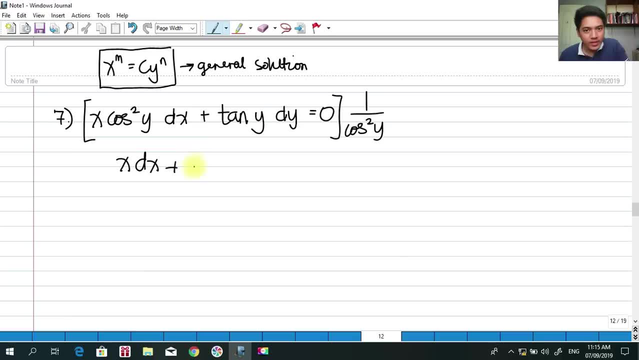 what will happen? we have X, DX, plus a tangent of Y over cosine squared Y. let me just rewrite this: okay, okay, so we have dy here is equals to zero, and again we need to integrate, they integrate. so what will happen here is that we have x squared over 2, okay, plus, as you can see here. 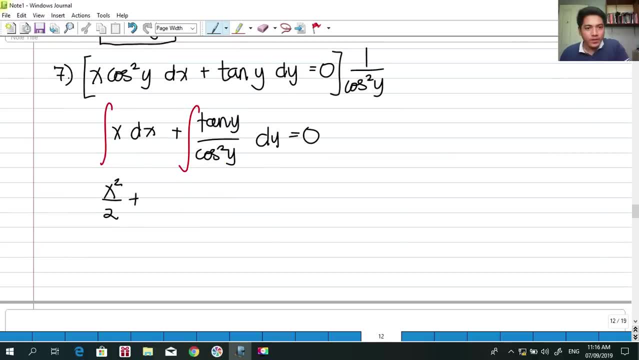 this is an integral of nine squared all over two. as you can see, here we have a higher integral by property or by trigonometric identity. one over cosine squared of y is equivalent to what? okay, if, if, uh, one over cosine theta is equal to secant theta. 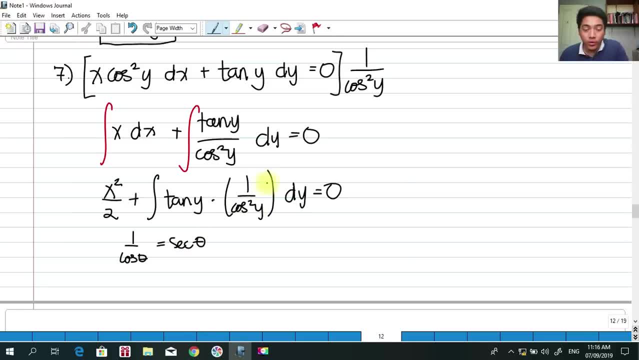 then this whole equation, or this identity, is now equal to what? so this is one half x squared equal to secant squared theta plus integral of uh. secant squared uh y, because our function here is y. okay, our function here is y, so we have secant squared y right times. tangent y dy is: 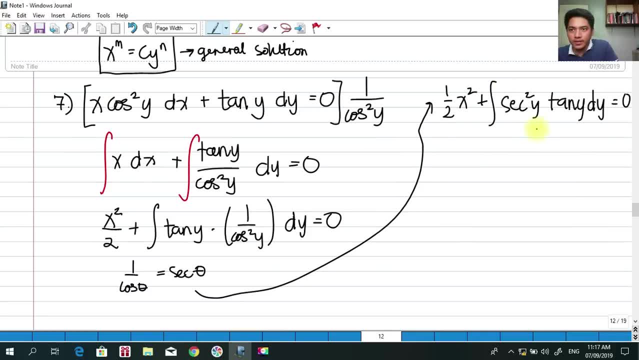 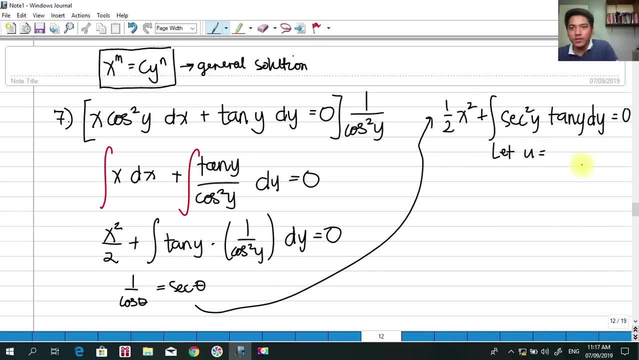 equals to zero. so how do we integrate this? how do we integrate this? we can integrate this by letting u as what? so in order to for us to to integrate this, we need to let u as tangent y du with respect to y is secant squared y du is now equal to secant squared y dy, which is available on our 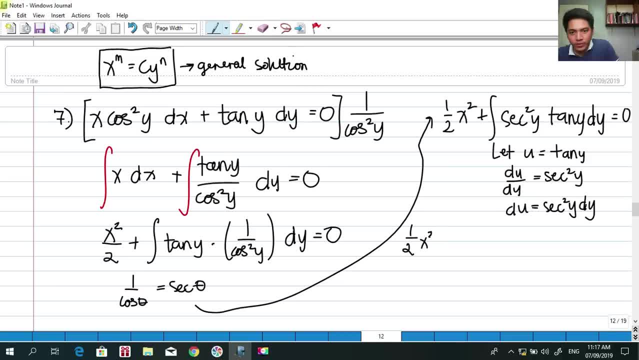 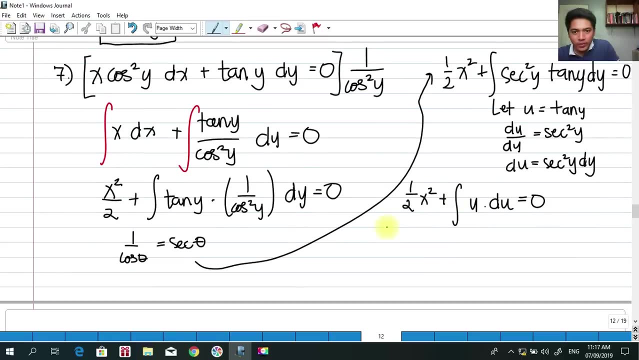 integrand so we have one half x squared plus. okay, the integral of again tangent y is u. secant squared y, dy is equivalent to du, equals to zero. so we have one half x squared plus u squared over two. again, plus c is equal to zero and we need to back substitute whatever the value of u. 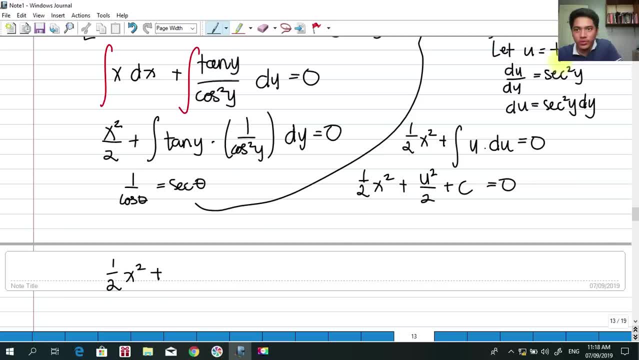 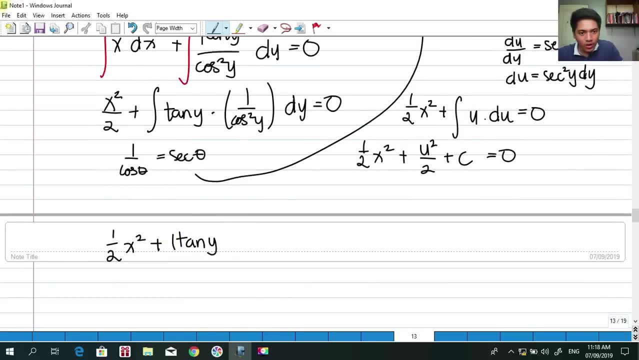 okay, plus what is u squared? this is use. u is our u tangent y, so it. it is now raised to two. okay, over two, plus again constants of integration is c. we can multiply this equation by two. we can cancel out one half so that we have x squared. 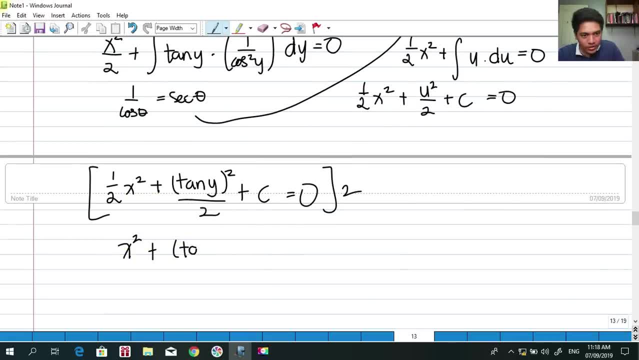 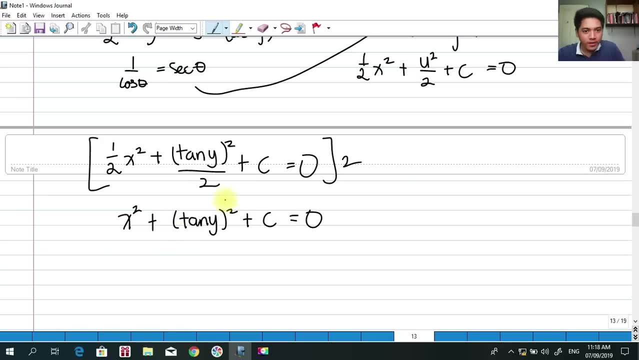 plus tangent of y, squared plus two times c is still c is equals to zero. and if we're going to distribute this, we have x squared plus tangent of squared y plus c is equals to zero. so this be our general solution for our problem, for this problem. okay, down to our last. 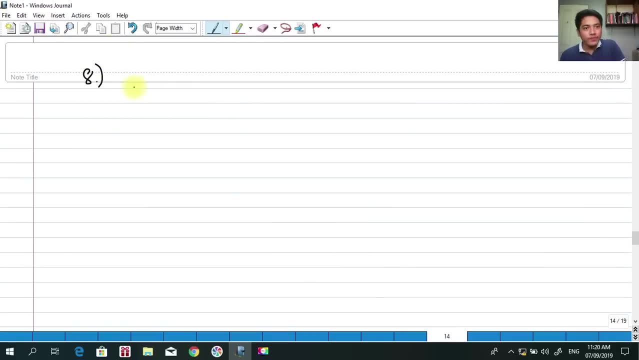 example for this video. so we have X plus 2. DX is equals to X plus 3, sine of Y, cosine of Y, dy. first step: again group them in terms of X and DX, Y to be Y, so we have. we can eliminate X plus 3 here, because this is purely Y, so we have X. 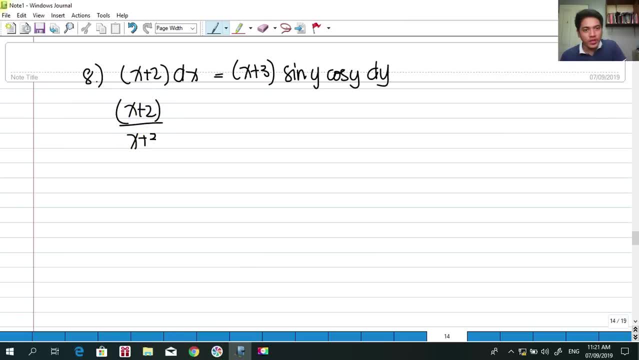 plus 2, by over X plus 3 DX, and this is now sine of Y, cosine of Y, dy, and we can now what integrate? okay, so, as you can see here, how do we integrate this first? so one factor is that we can always make the numerator the same as the denominator, given that if we are only have to add, 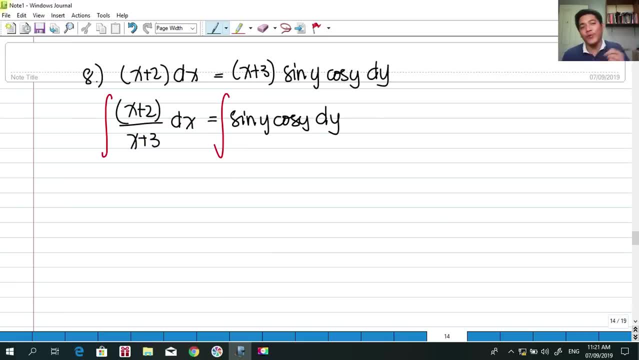 constant. we cannot add X terms here or Y terms here, so I'm going to rewrite this equation as X plus 3, okay, X plus 3 minus, let's say, X plus 3 here. this should be X plus 3 minus 1, so we have DX, okay, and. 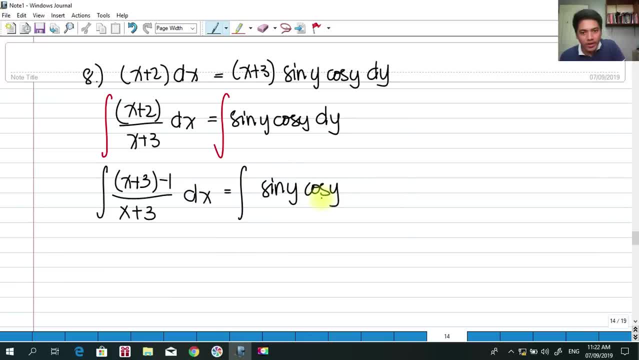 integrating this sine of Y, cosine of Y, dy. so this is a, this sign of Y and cosine of Y has a relationship with each other, so that if we left U as equal to sine of Y, Then the du with respect to dy is cosine of y. 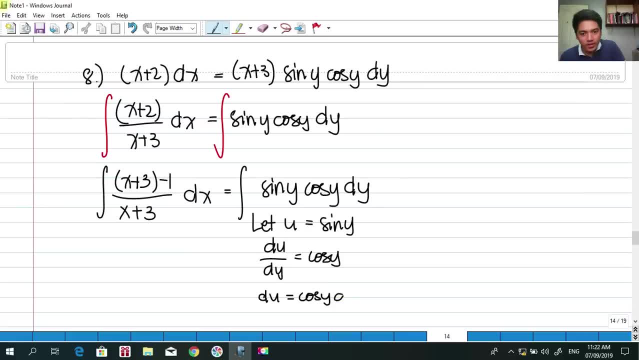 Cross-multiplying we have: du is equal to cos y, dy, which is readily available. So this is simply a u-substitution, But in here we can still perform the property of integral, wherein we can substitute or distribute the integral and dx sine. 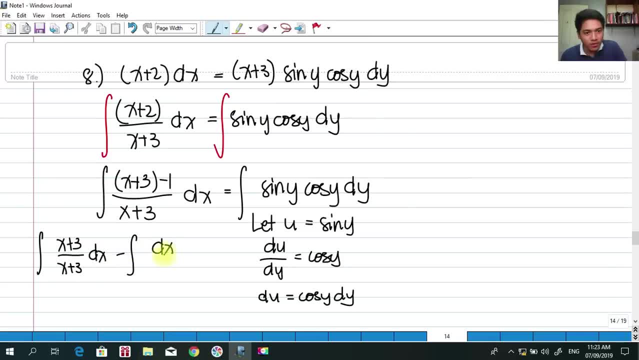 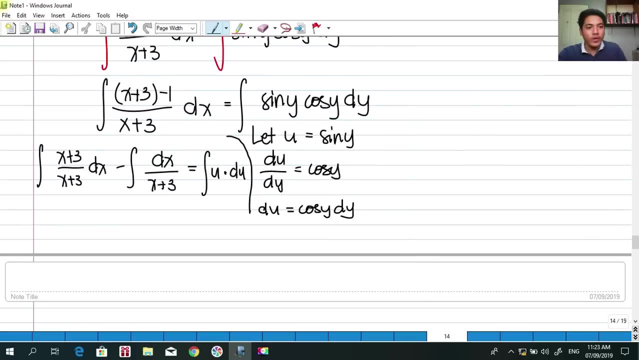 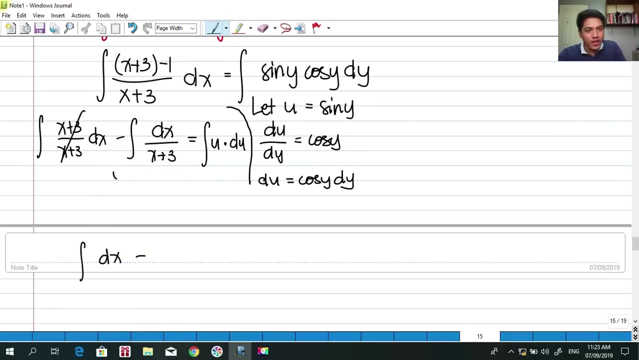 So we have minus dx over x plus 3, and that is equivalent to the integral now of: if we let you assign y, u, then du. Okay, so we can see here that this should cancel. So what will happen? we are left with dx minus. okay, if we let u here as x plus 3,. 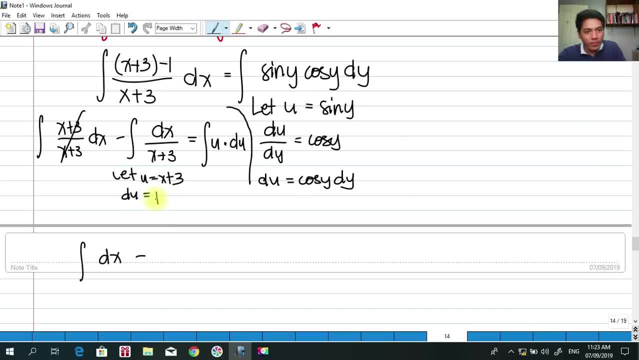 du with respect to x is 1.. Okay, multiplied by dx is simply dx. So simply, you are left with this. dx or du over u is equal to integral of u times du. Okay, so here, simply, this is still ln okay because du over u. 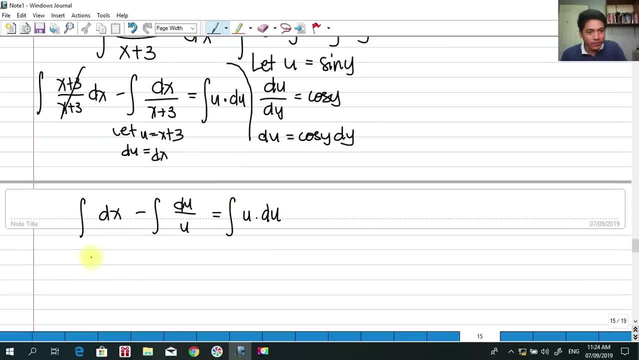 So what will happen? We have what Integral of dx is x minus ln of u. This is u squared over 2 plus c, but u here is equal to x plus 3, and the u here is equal to sine of y. 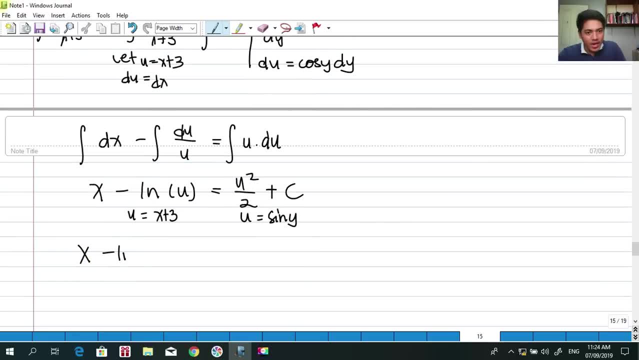 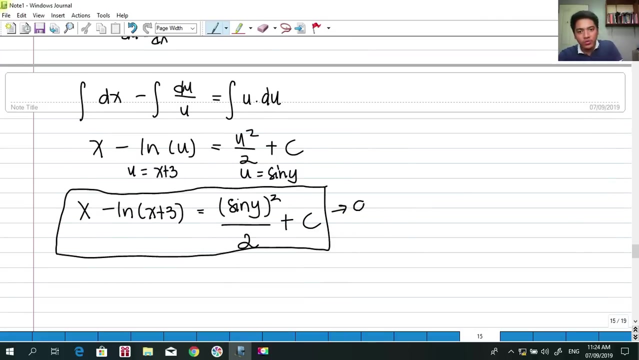 So we have now: x minus ln of x plus 3 is equal to sine of y squared over 2 plus c. Okay, So this should be our answer. okay, for our last problem. This is a general solution, since we are not given any condition. okay. 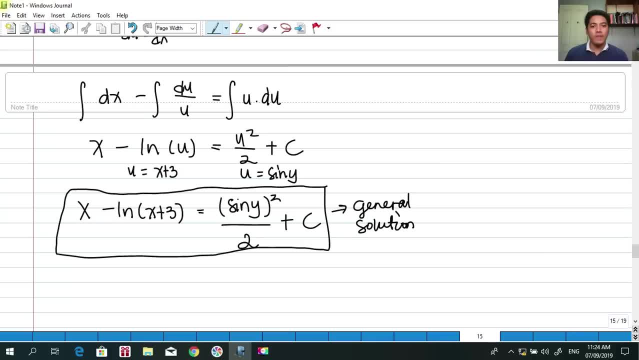 So that's all. Thank you so much for viewing my video. So this is Engineer Abba. This video is all about the variables, the parable of D, and I hope you learned something today. Thank you so much, and God bless you.